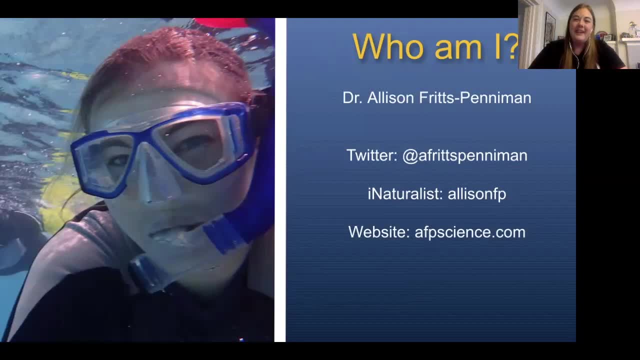 And you can find me on Twitter at a Fritz-Penniman, Or on iNaturalist with the username AllisonFP, And if you're not familiar with iNaturalist, I highly recommend it as a place to learn more about the natural world around you. 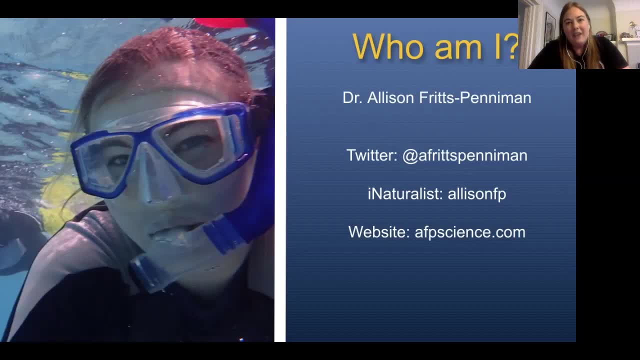 It's a website for uploading observations of organisms that live that you see wherever you are, And it is also a social platform to where people can help each other identify species and, you know, meet each other over the internet, which is great in the time of staying at home. 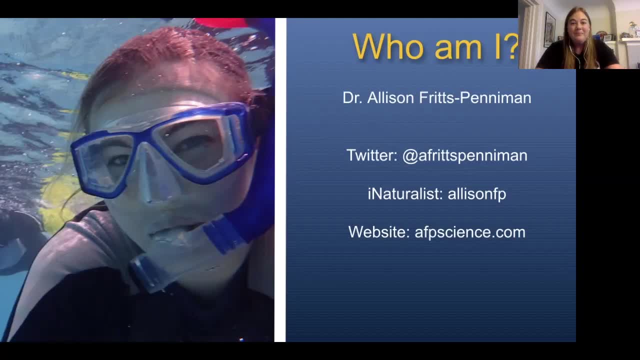 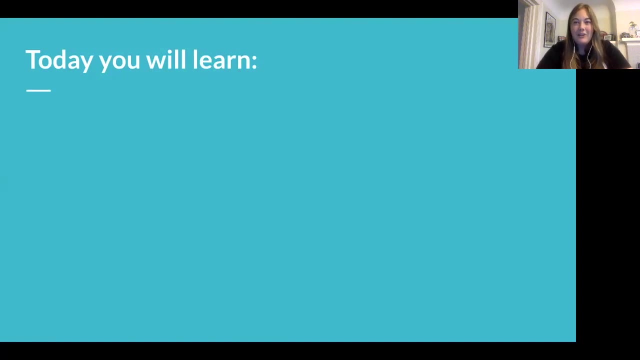 And then I also have a website, AFPSciencecom, And I'm happy to be. I'm happy to hear from any of you and answer questions, And I'm also a part of the Facebook group for marine biology at home. Today, my goals for you are to learn that corals are amazing creatures. 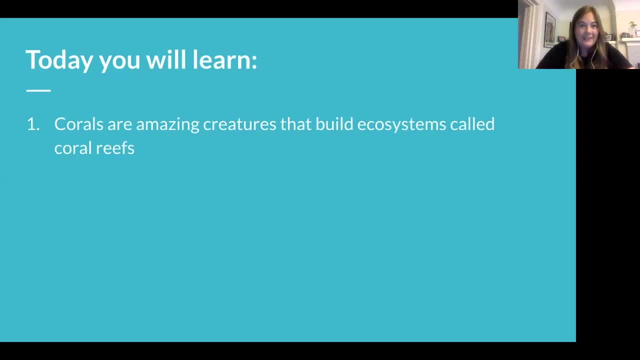 That build ecosystems called coral reefs. Obviously, that's the topic of discussion today. Coral reefs are biologically and ecologically diverse. They are highly threatened by human activities And we need to conserve them. And there's a lot of research to be done. But as we proceed, we need to make sure. 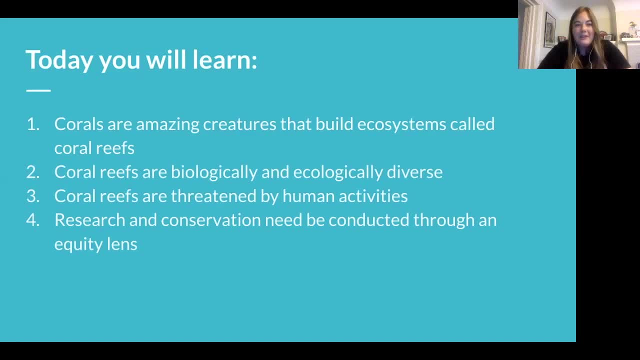 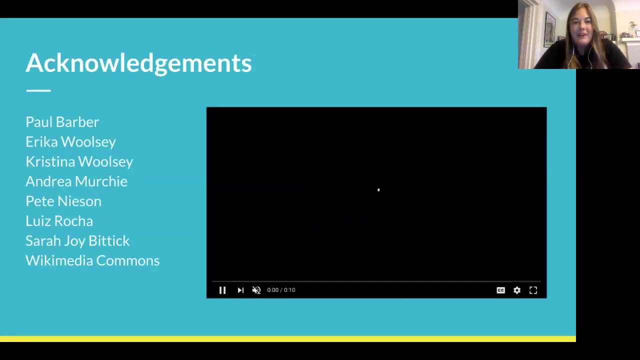 That we're approaching this work Through an equity lens, And so I'll finish talking a little bit about that Before I get going. I just want to acknowledge some of the people who have informed this lecture today, starting with Paul Barber, my dissertation advisor from grad school. 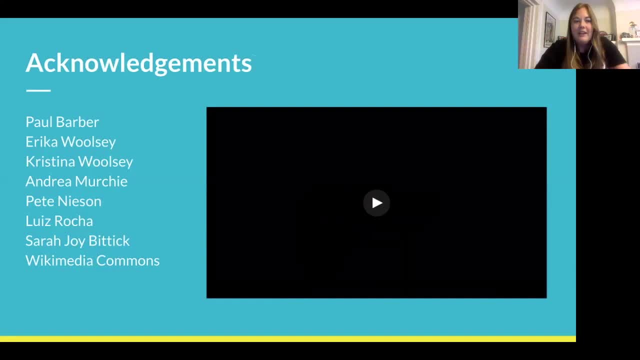 Some of the slide info and, like the general outline of the lecture I can attribute to him. And then this organization, the Hydris, That I is a nonprofit that I worked with in San Francisco, And several of the individuals that I worked with contributed photos that I've used in this talk, also design elements for the, the lecture as a whole, And then also I used a few photos from Luis Rocha, Sarah Joy Biddick and Wikimedia Commons. 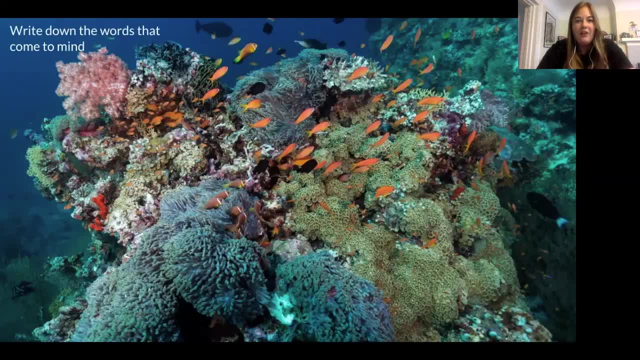 But it says right here, and then I have two others here. All right. so I want to start out by Just getting the feel of coral reef. Now, this is maybe a little different from your typical science lecture, but this photo, And if you need to pause the video while you're- 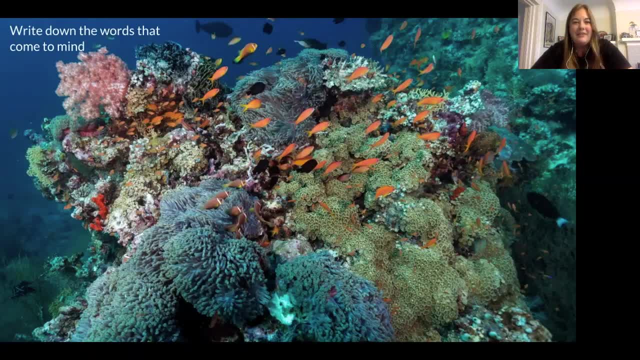 writing. please do so anytime. Remember this is: I want this to be an active learning experience, not just you watching a video here. So I'm going to show several photos and I want you, for each one, to write down what words come to. 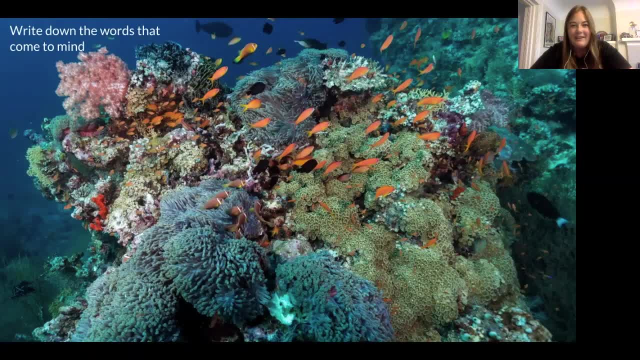 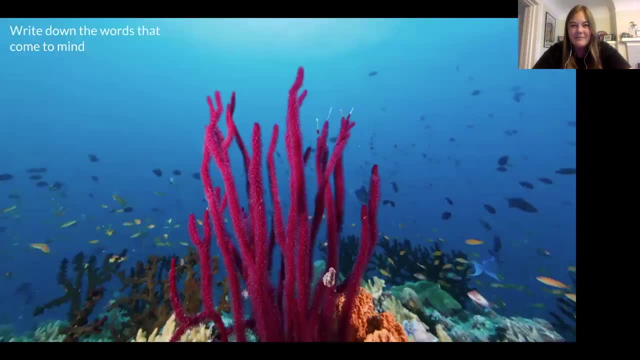 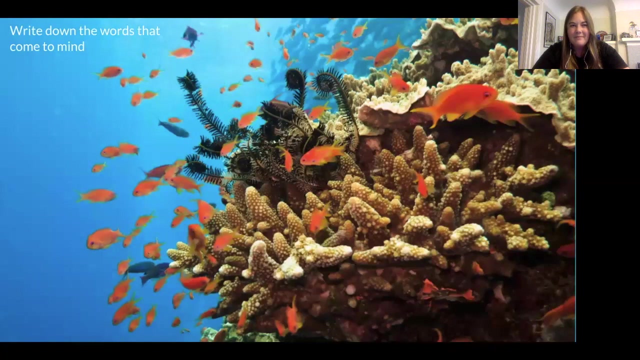 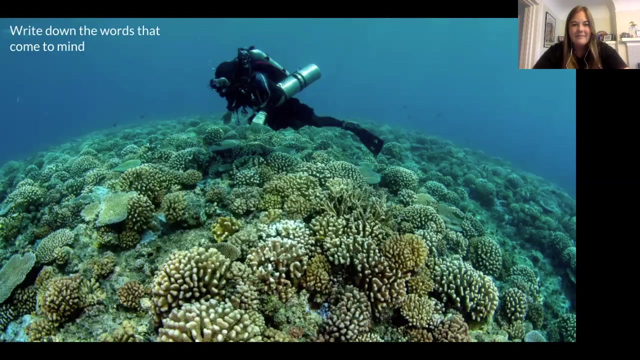 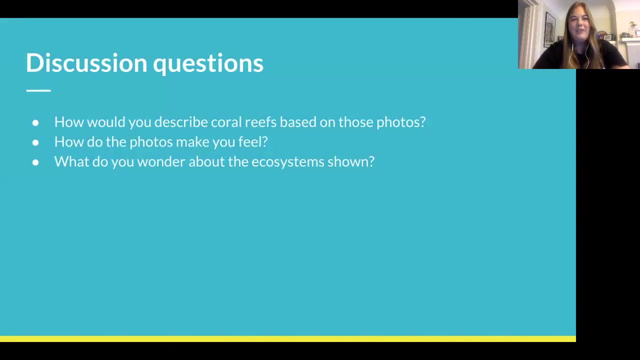 mind And remember. yeah, you can pause at any time to spend more time on these photos. Okay, I'm going to move on to the next photo, All right. next photo And the next photo. Okay. so when you've taken some time to look at each of those, 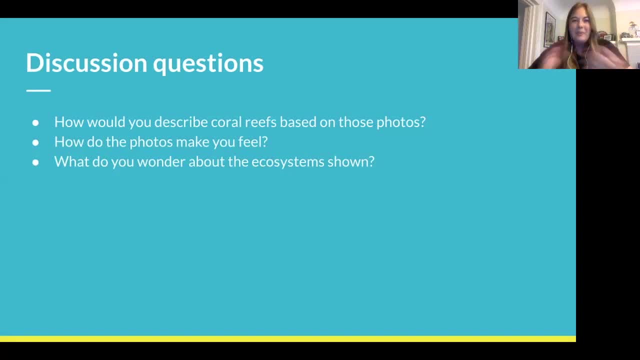 photos I want you now to summarize in, either in discussion, if you are working through this lecture with another person, or in a journal, to please describe coral reefs based on the photos that I've shown you. So, just based on that look, basically those four photos. what can you? 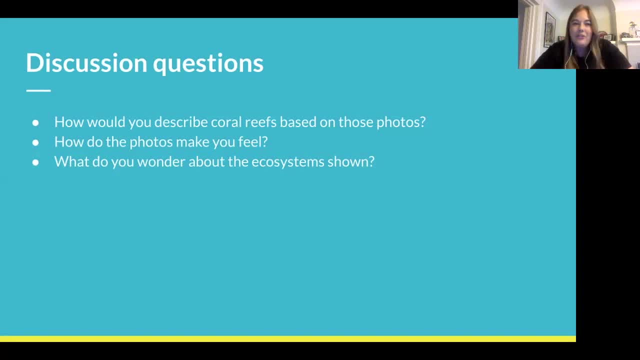 say, about coral reefs, And I also want you to describe how the photos make you feel. And if you've watched the other lectures from this marine biology at home series, you'll know that one of them talked a lot about values, And that was the. 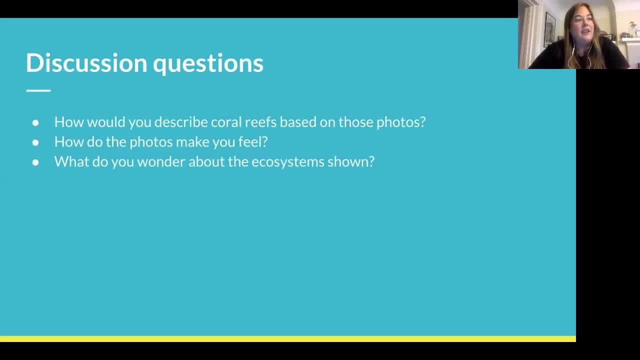 conservation lecture And so values take. they play a huge role in our conservation attitudes and actions, And so describing how these photos of coral reefs make you feel is connected to your values relating to coral reefs, And that's why I'm asking you that question. 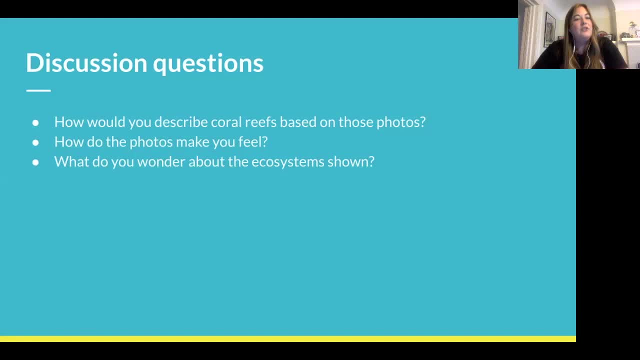 And then, lastly, I want you to write down what you wonder about the ecosystems that are shown And hopefully I'll answer some of those questions throughout this lecture. But if not, these are some questions that you may want to ask in the Facebook. 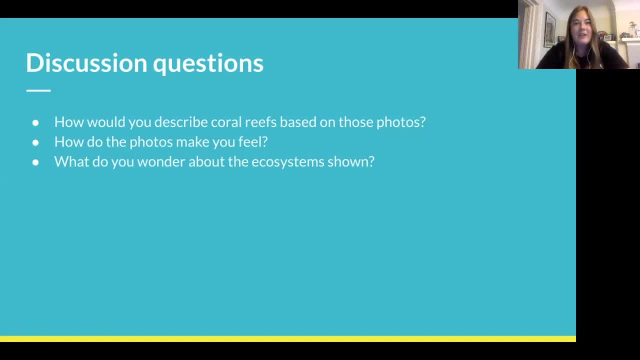 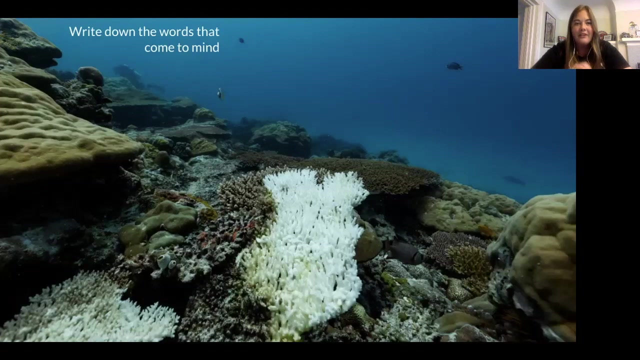 group, So take a few minutes to answer these questions before moving on. All right, so now I'm going to show you another set of photos, And it's the same exercise. I still want you to write down the words that come to mind as you look at these photos. And again, 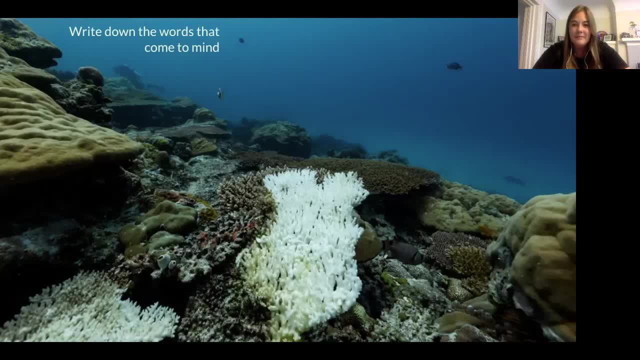 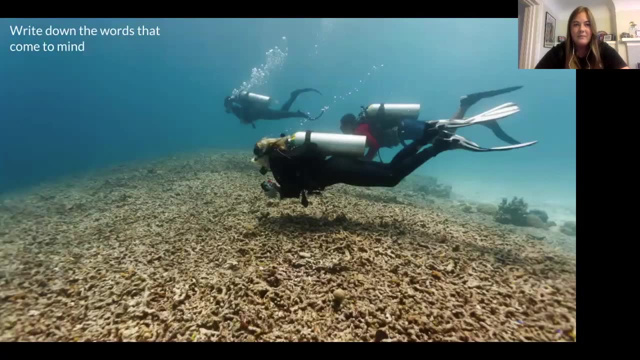 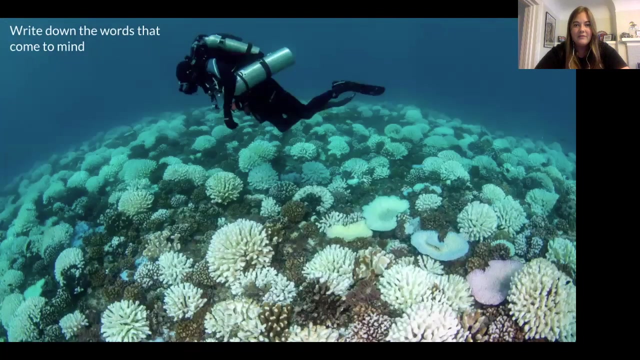 remember: pause at any time. Okay, next photo And next photo. And please do write down what words you're thinking of, because the act of writing down what you're seeing and thinking is a really important part of the learning process When I was a 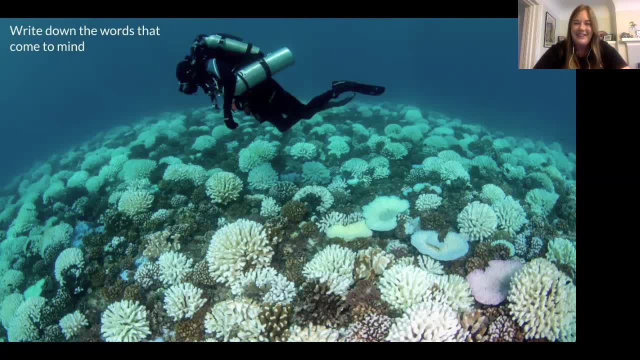 student. I used to just cut corners a lot and not really take notes, just think I'm just I'm going to remember all of this, But I regret that now. I wish I had taken more notes and spent more time reflecting on what I was thinking and 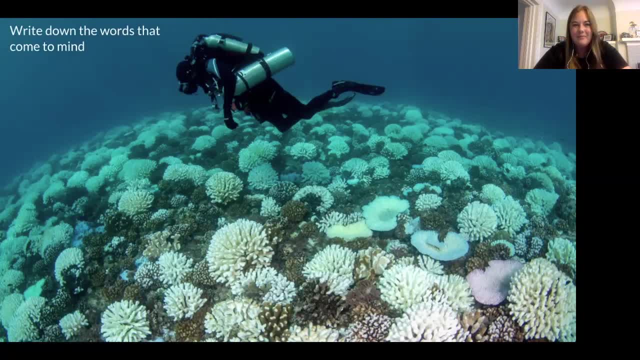 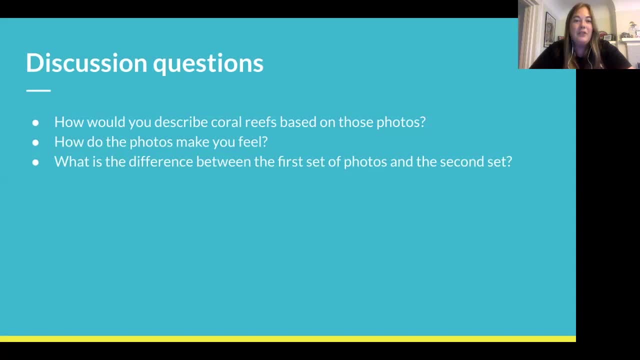 learning. Okay, so once you've looked at those photos, I have the same. Okay, so once you've looked at those photos, I have the same. Okay, so once you've looked at those photos, I have the same questions for you. How would you describe coral reefs based on? 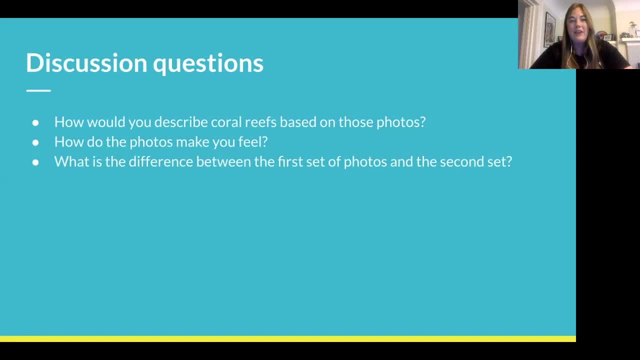 just those last three photos. How do the photos make you feel And what is the difference between the first set and the second set? Got my cat here joining us. Tried to lock him out, but he he can open the door by himself, So didn't really. 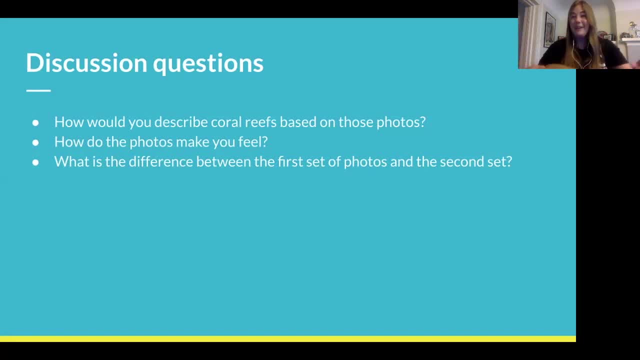 work out. This is my cat, Milo. Hopefully his purring isn't too loud, Alright, so yeah, pause the video and take some time to really think about how you would describe the difference between the first set of photos and the second set of photos. 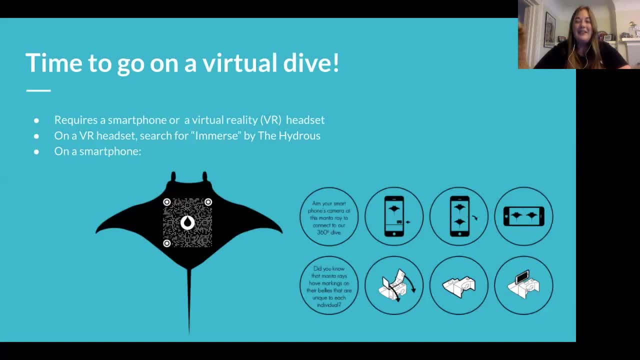 Okay, so once you've done that, I'm going to take you on a dive, And you don't need to go to the ocean for this dive, you just need to take a smartphone, If you happen to have a virtual reality headset. I don't have one, But if you have one, you could also. 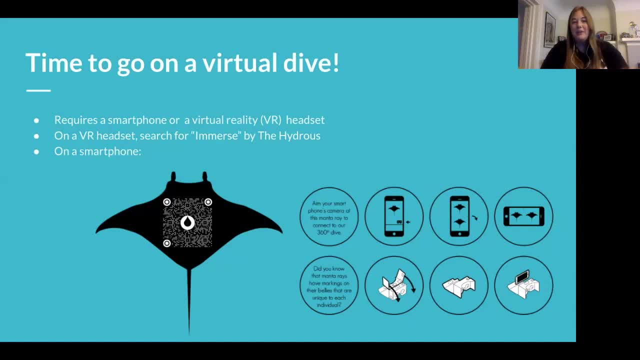 watch the video there If you search for immerse by the hydris. But the easier way to do it is on a smartphone. So pause the lecture And what you'll do is take your phone, open up the camera app, Hold it up against the QR code. 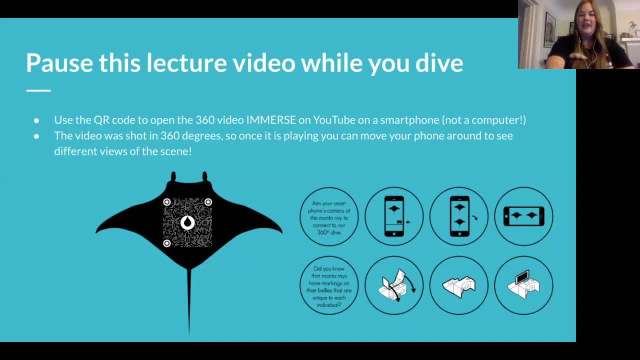 That's on the manta right here, And your phone should prompt to open the YouTube app And it will open this video. the video was shot in 360 degrees with a special 360 camera, So the cool thing about watching this on your phone is you as you move. 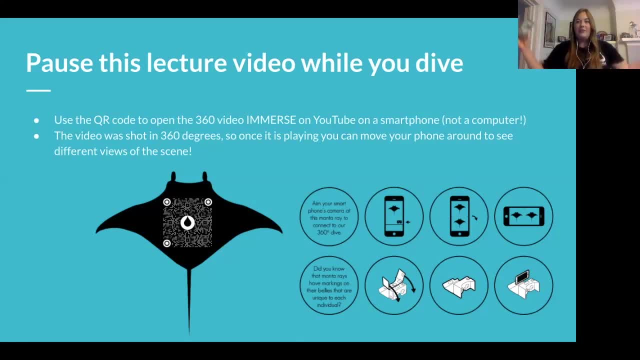 your phone around. it'll show you different views of the 360 degree scene. So don't just watch it like this, Watch it like this. this stand up, turn around Really, really try to see the whole scene around you And this. 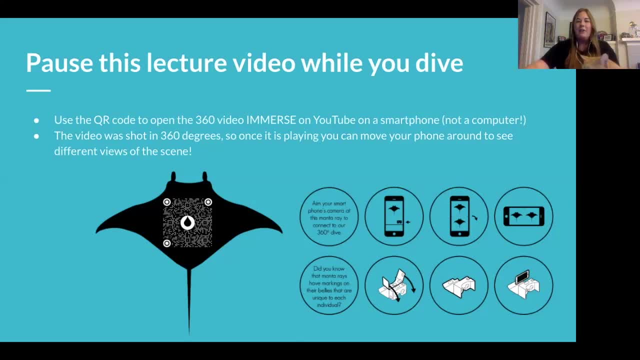 video is about nine minutes, So make sure to pause this lecture while you watch that. And this is just an opportunity to really immerse yourself in a coral reef and learn more about the ecosystem and some of the threats that that they face. Okay, so after you've watched, immerse, you're going to want to. 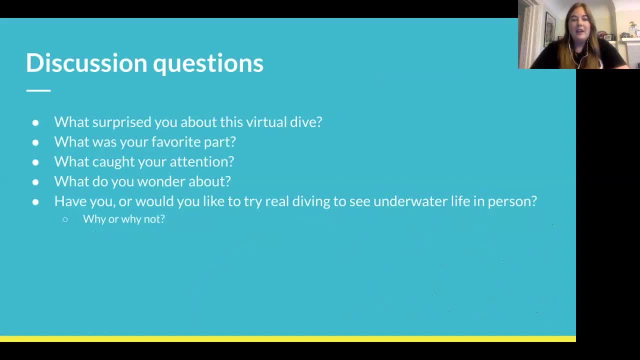 watch the next video. Please take some time to either discuss these questions with another person who also watched it, or journal about these questions. So what surprised you about this virtual dive? What was your favorite part? What caught your attention? What do you? 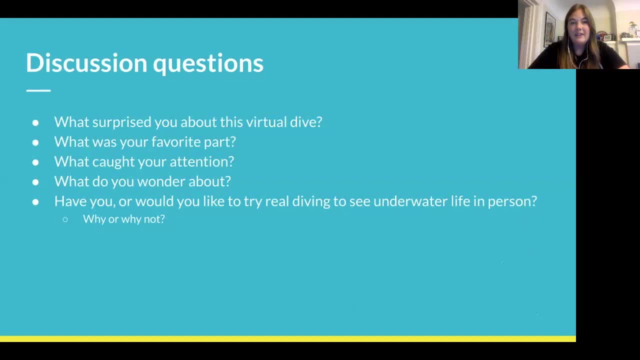 wonder about. Have you ever been diving? Would you like to try? Why or why not? So again, pause the video. Take some time to answer these questions before we move on. Alright, so after you have journaled about the video, come. 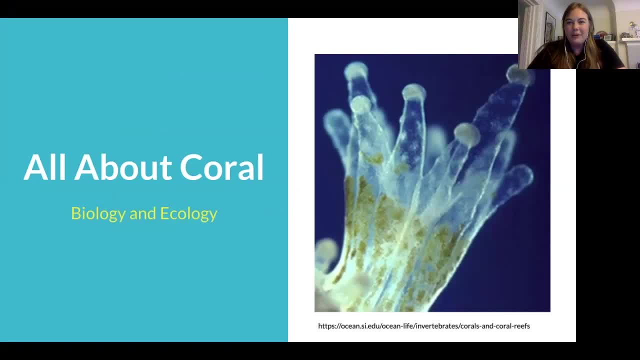 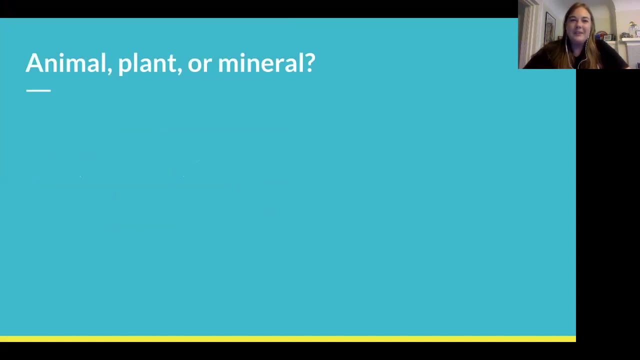 back and we will move on to all about coral. So in this section I'm going to talk about some coral and why or why not coral, biology and ecology. and I want to start with a question: do you think coral is animal, plant or mineral? so pause for a bit and just think, come up, decide on. 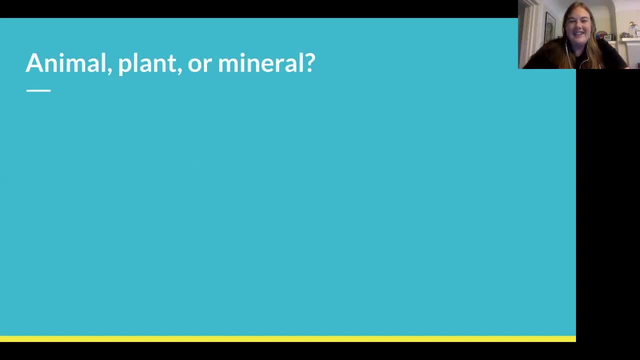 an answer you already know. great, if you don't give it a good think before we move on. all right, so it's a little bit of all three, but technically, taxonomically, corals are animals and they're in the phylum Cnidaria, along with jellyfish and sea anemones. 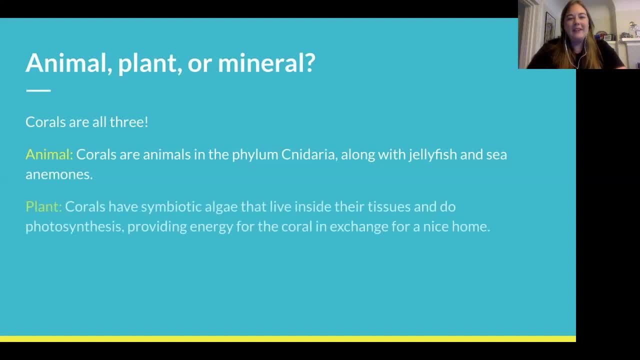 the reason they could be kind of considered plant-like is that they have symbiotic algae and they're in the phylum Cnidaria along with jellyfish and sea anemones. the reason they could be kind of considered plant-like is that they have symbiotic algae. 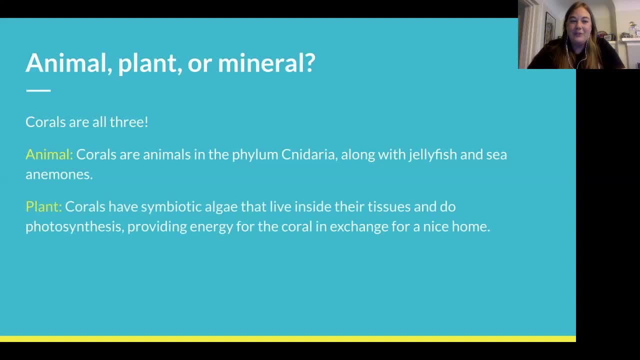 that live inside their tissues and do photosynthesis, providing energy for the coral, and in exchange, these algae get a nice place to live. and so these algae- while you know, algae and plants are different kingdoms of life, but they have a similar photosynthetic system. so when corals have these algae living inside, 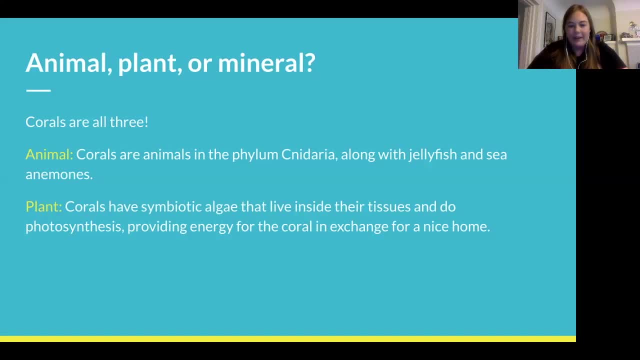 them doing photosynthesis. it does make them kind of plant-like and they also look a little bit plant-like. you know, if you are used to seeing plants around you on earth as your typical, you know structure providing habitat, then corals are sort of like the equivalent under 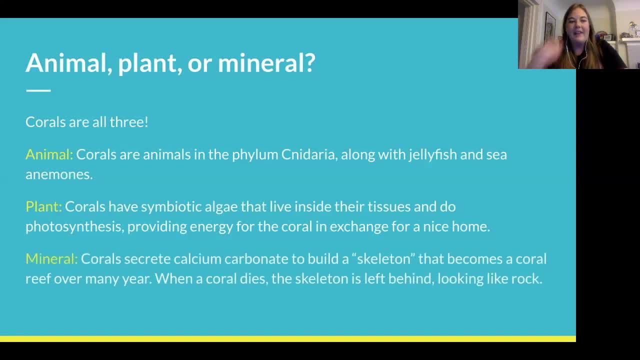 water, and then the mineral part is the fact that coral secretes calcium carbonate to build a skeleton that is left behind even after a coral dies, and so it they basically do produce rock in a way, although I kind of like to think about how you know if you think about a human skeleton that's left behind after we die. 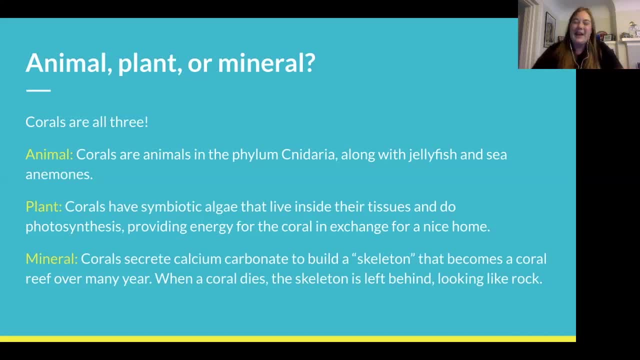 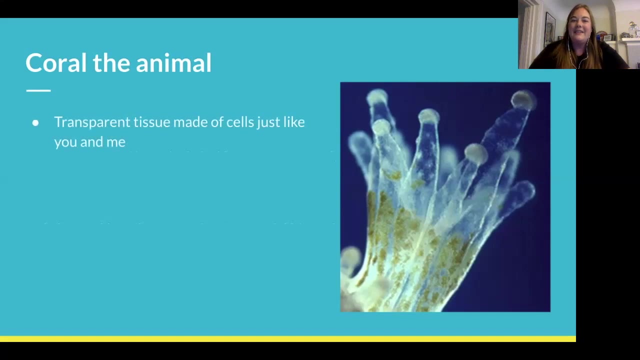 as well, so you wouldn't call us rocks. so you know, just food for thought. but there's our components to corals that are animal, plant in the know. so coral the animal is actually has made up of transparent tissue and the cells are the same type of cells that we have as humans, except that they have these. 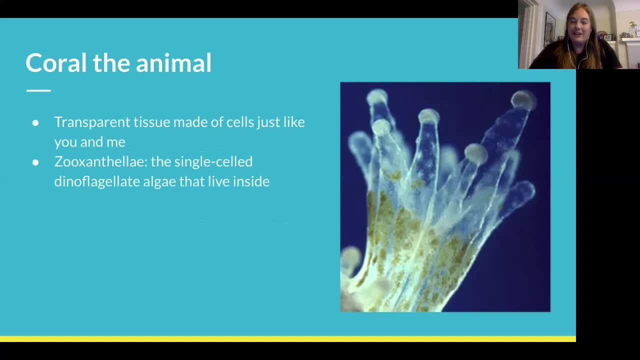 zooxanthellae, the single-celled algae that live inside of their cells, and in this case we have a single-celled algae that live inside of their cells and in this photo they appear greenish brown, but they can also be other colors and this: 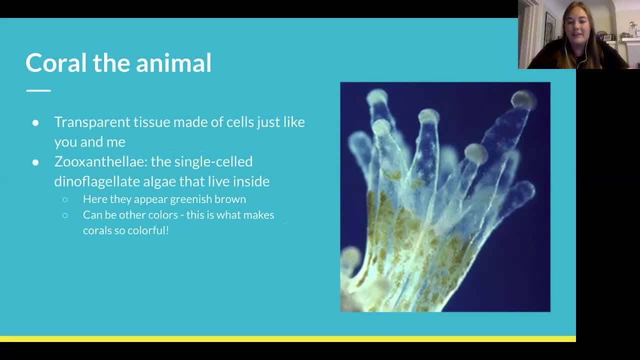 is what makes corals so colorful, is the zooxanthellae that live inside of them. and this is an example of a symbiosis, which is when two species form a close relationship and often that relationship involves living together. in this case, it's a mutualism, because both species benefit from that partnership. 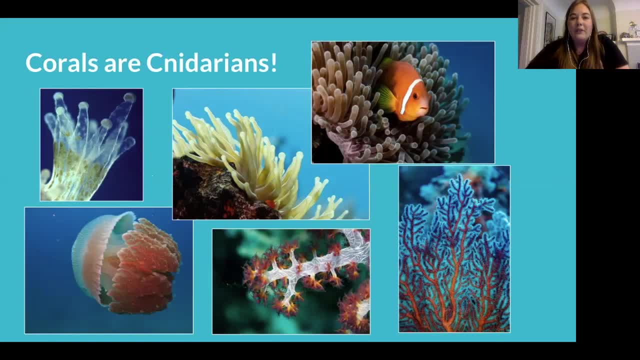 so sometimes they have different opportunities and that rose or even dying, is a mutualism. so, with all this being said, this on the upper left of your screen, we actually have two pictures on here. these are two images of the Eurasian and the Eurasian blue corals which you can see here are one. 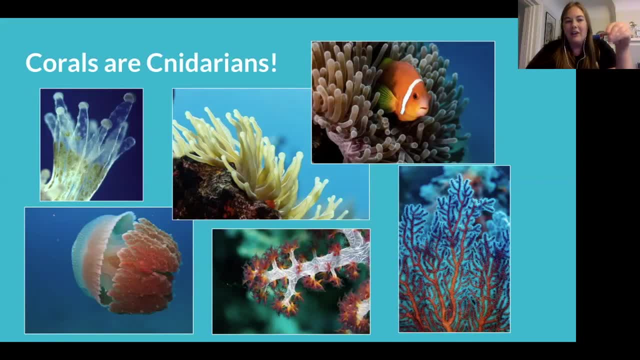 by one. so we have this one by one and then this one by one, and then this one, and then this one by one, and this one by one and then this one by one. so if we look at the picture in the image, you'll see that these are different things. 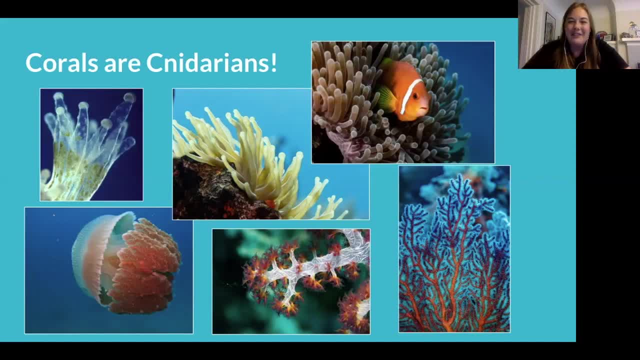 And anemones are famously the homes of Clownfish like Nemo- We actually just call them anemone fish in the marine biology world- And jellyfish, like on the lower left photo, also have tentacles. And then these other two photos are of soft corals where the tentacles 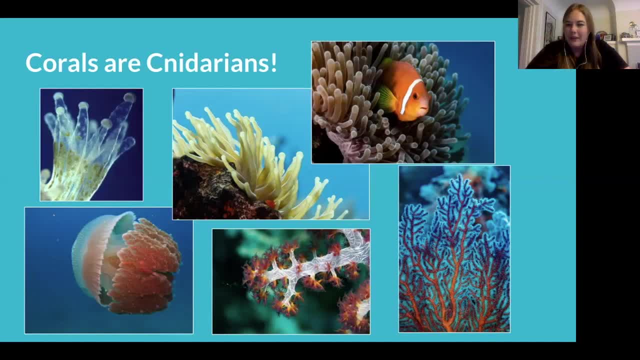 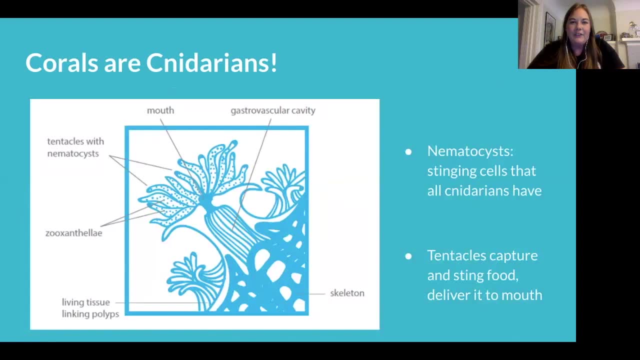 you can actually see pretty well even without zooming in close. So those tentacles are something that Cnidarians all have in common And if we look at a diagram of a cross-section of a coral polyp, you see it's got the tentacles which have nematocysts and zooxanthellae. 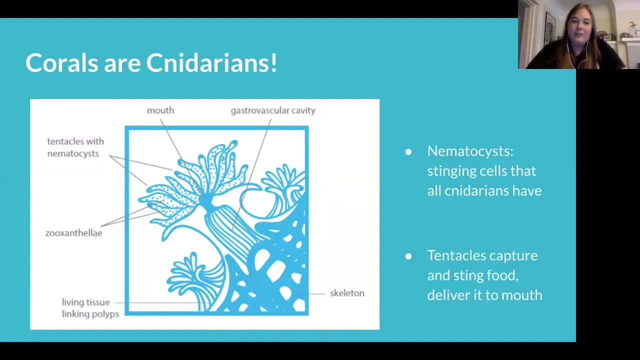 And they have a mouth in the middle which leads down to a gastrovascular cavity, And then they have this skeleton underneath And so they secrete that calcium carbonate um along the bottom of the polyp and it builds that coral, hard coral structure. 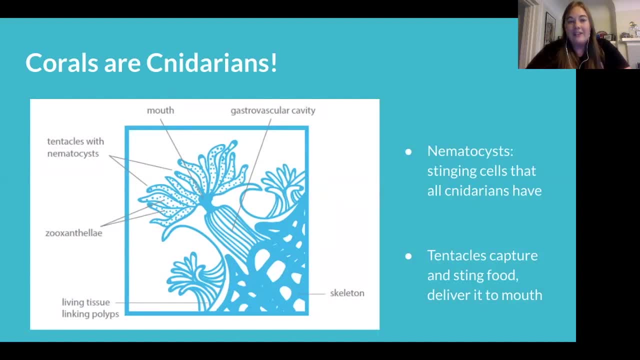 The nematocysts are stinging cells that all Cnidarians have in common, And so the tentacles have those nematocysts and they can capture food and bring it to the mouth, Kind of just like us Um, and then it will be digested in the gastrovascular cavity. 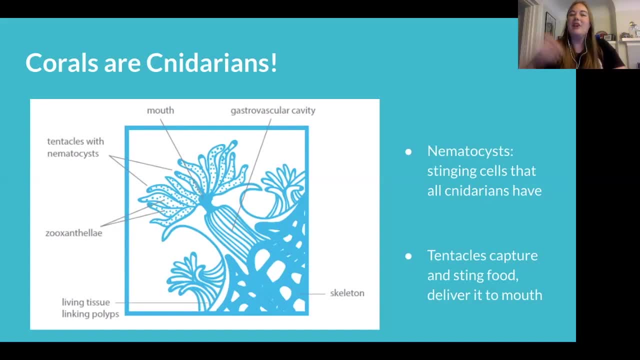 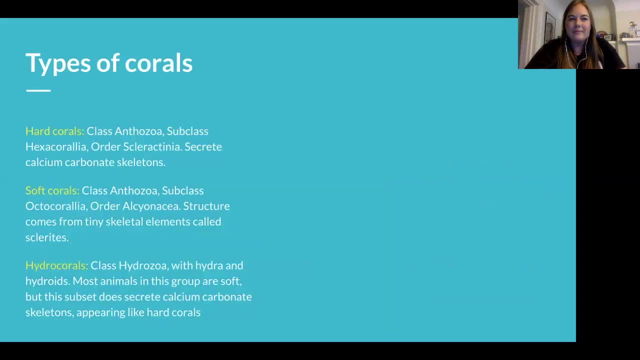 So they're getting food from the zooxanthellae, but then they're also getting food that they've captured out of the ocean water. Okay, so now I'm going to go through the three categories of corals, And the first is hard corals. 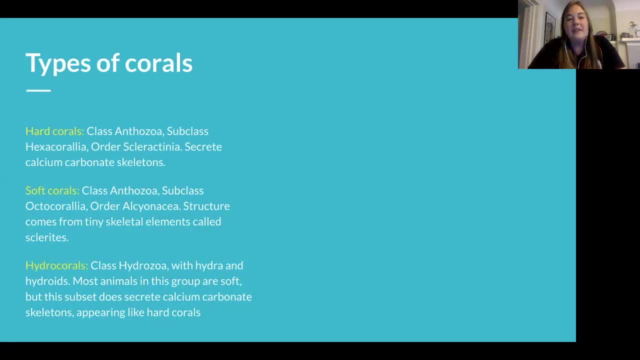 And so these are in the class Anthozoa, subclass Hexachorallia and order Scleractinia, So we would call them Scleractinian corals, And they secrete calcium carbonate skeleton, and these are the more. this is the type of coral that you. 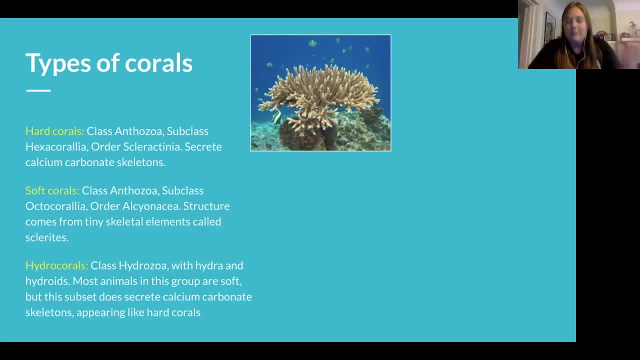 you probably picture when you just hear the word coral. They have these hard skeletons. Next category is soft corals, And these are in the same class, Anthozoa, So that that class is what we call the true corals. Then they're in the subclass Octochorallia. 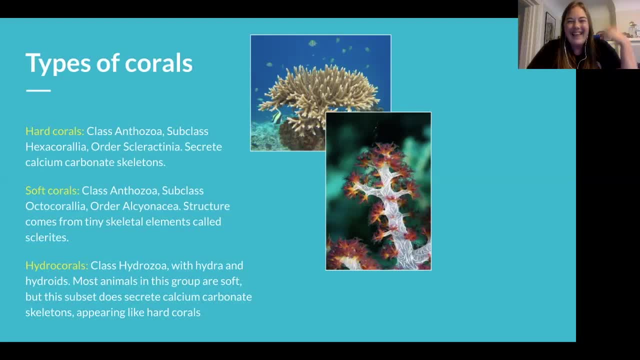 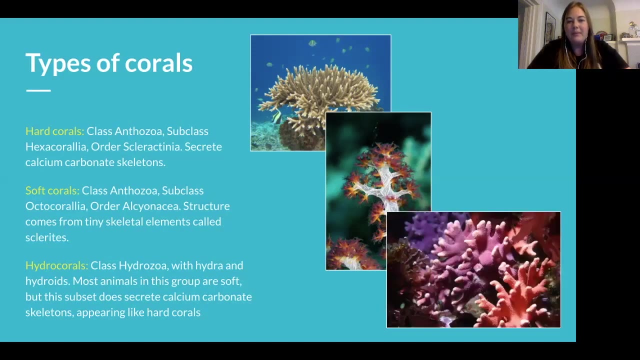 and the order Alcyonacea, And Okay, And their structure is not from a calcium carbonate skeleton, but instead these tiny skeletal elements called sclerites. And the third group is called Hydros Hydrocorals, and they're not in the true coral group. 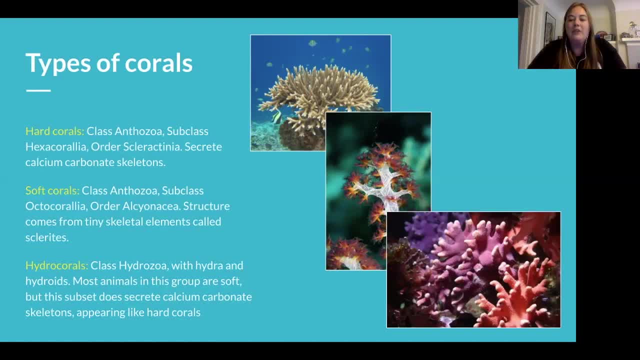 They're actually in class Hydrozoa, which is the same class that Hydra and Hydroids are in. It's a different type of Cnidarian And most of the animals in this group are soft, So, Hydroids- they look even more like plants, to be honest. 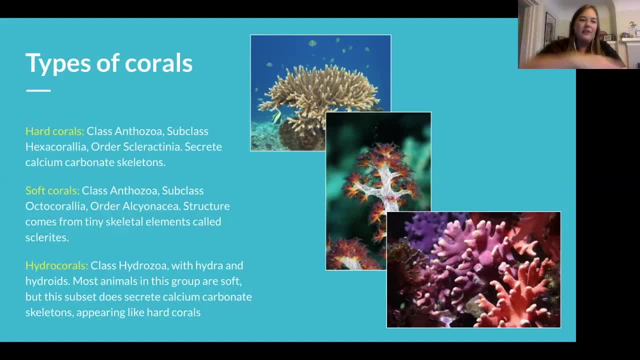 They're very, you know, they're always flowing with the current and you have to be careful because if you do, if you run into them, they'll really sting you, more so than corals do, And they, these specific subset of Hydrozoa, does secrete a calcium carbonate skeleton. 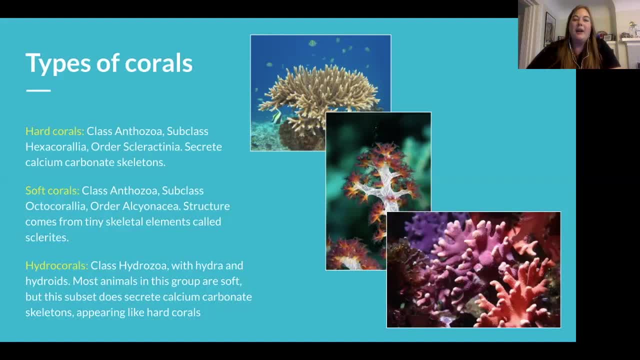 So They look like hard corals And that's why they often are called corals, Even though they're not in the same class. So you can see how taxonomy is important, because it helps us understand how species are related to each other. 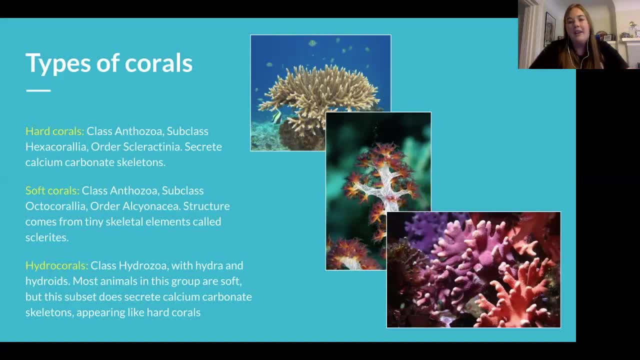 But structure and function is also very important When it comes to putting these species in context in their environment. So Hydrocorals play a similar role in the ecosystem That Corals do, And they appear similar, So a lot of people will kind of categorize them as corals, even though taxonomically 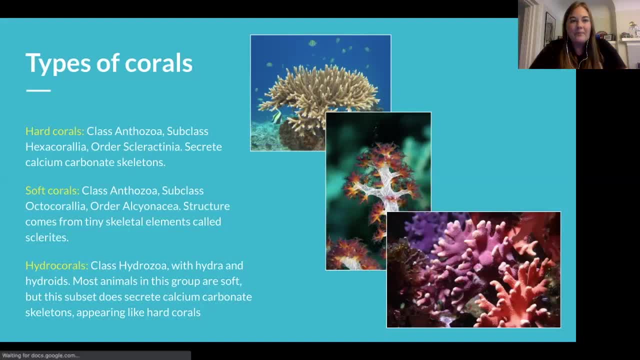 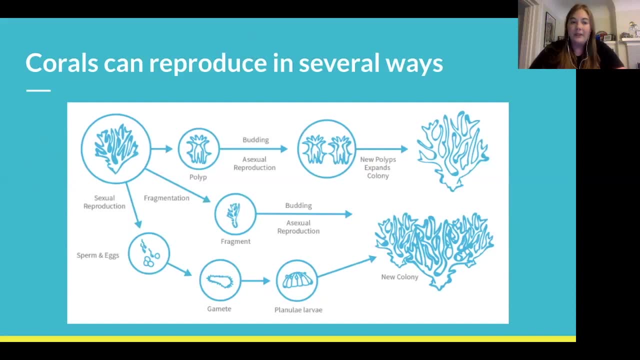 they're different. Corals can reproduce either asexually or sexually, And so this diagram shows three different modes of reproduction. The top two are both asexual, And then The bottom path is sexual, So the asexual reproduction is through budding. 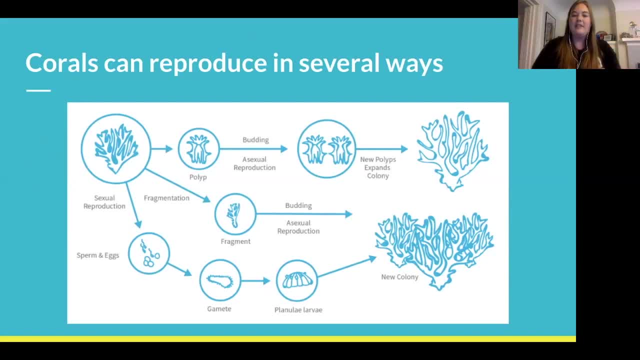 And this is how colonies grow. So the very top path on this diagram is just showing how, when polyps split, new polyps are formed and the colony itself expands. And corals like this. the coral organism is colonial because it has these identical 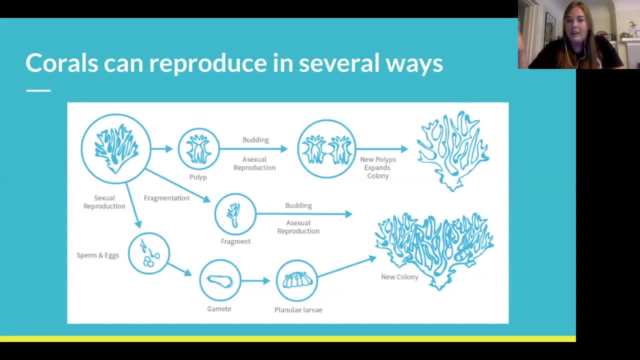 polyps, So the individual coral. you could say that each polyp is an individual and is reproducing to produce. you know these daughter polyps. But it's also okay to say that the colony itself is an individual, because the colony is they're. they're secreting calcium carbonate into one solid colony structure. 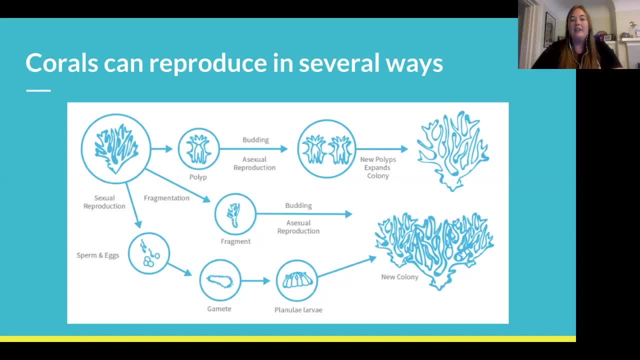 Now New colonies are formed in through the other two pathways, So either a fragment of a colony breaks off and attaches to a substrate and then buds and grows, Or corals also do sexual reproduction, And so this is where corals will produce sperm and eggs. 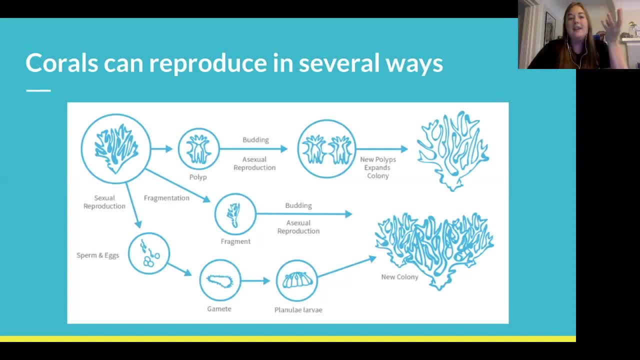 So each little polyp will will release either sperm, eggs or a combination of both, And then They end up Fertilizing In a column, Forming larvae and settling and growing into new colonies, And sexual reproduction creates genetically unique individuals, whereas asexual reproduction 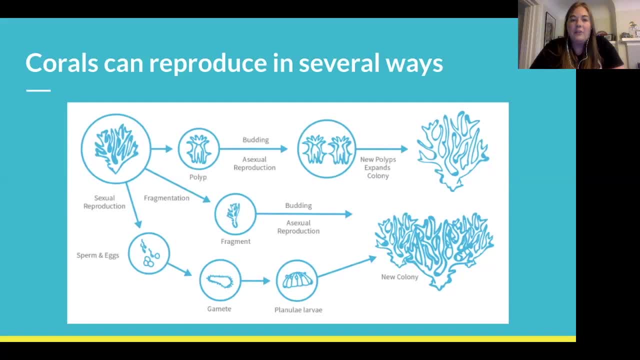 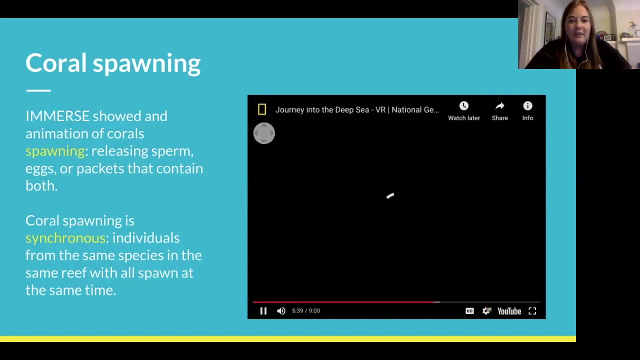 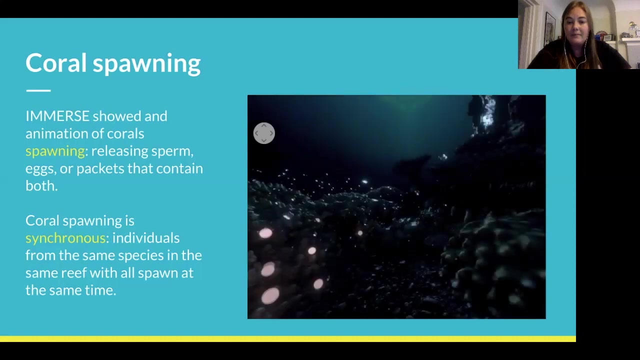 produces clones, So sexual reproduction is really good for introducing genetic variation into the population. Now, hopefully you remember In The immerse Film There was this part that actually showed Corals can replenish themselves through mass spawning events each year, when billions of 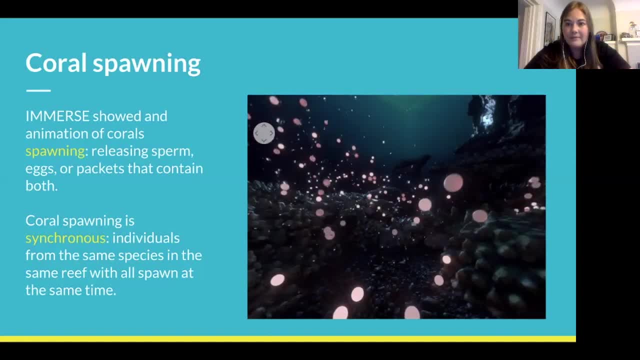 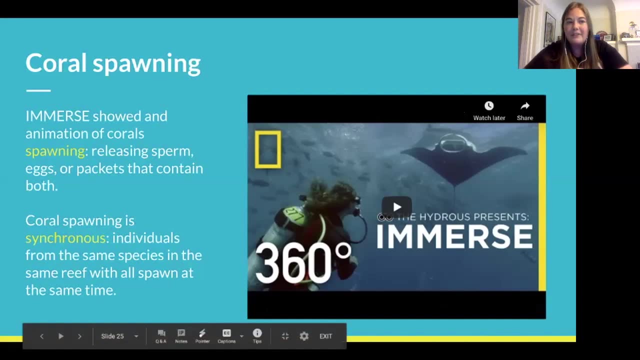 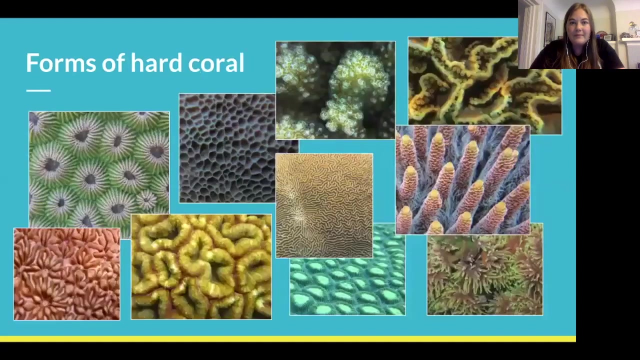 gametes are released after sunset and around the full moon, So that clip showed corals spawning and The corals spawn in a synchronous way, So individuals From the same species in the same reef will all spawn at the same time And that increases their chances of successfully fertilizing each other's gametes. 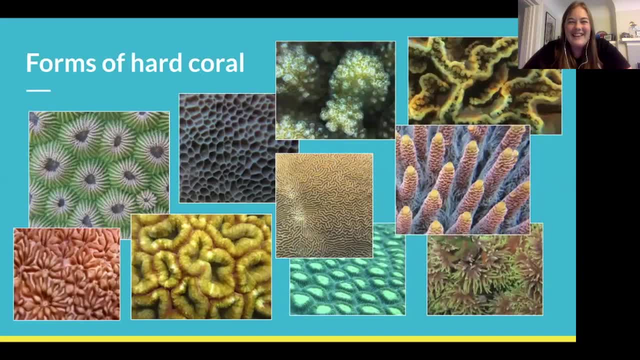 All right. So this is one of my favorite slides. This shows the diversity of The sort of microstructure that corals can form, So different types of corals have different shaped Coral Polyps, and like which is the skeletal structure of Apollo. 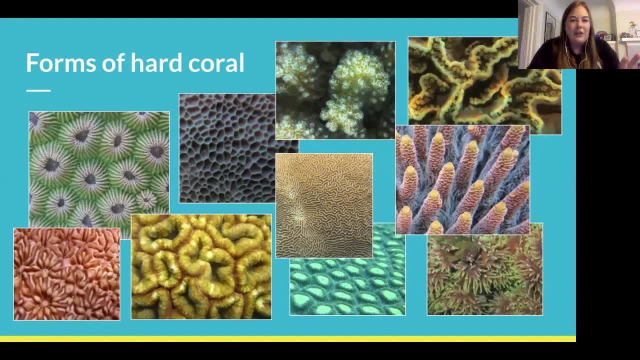 And so this ranges from The kind of large correlates that you see on the left side Of this- these photos- to the very small correlates In the upper right Photos And the- And I don't have a scale on these photos, But 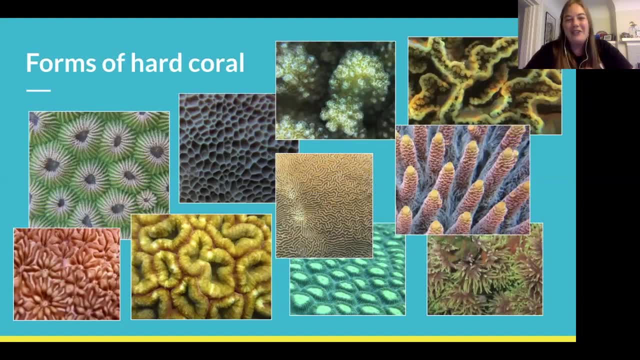 I'll just tell you, Yeah, of these, I know for sure that the ones on the left are quite large. you also have polyps, such as the bottom right, where there's very long tentacles sticking out. so certain species of corals will either have their tentacles out during the day or during the night. it depends on when. 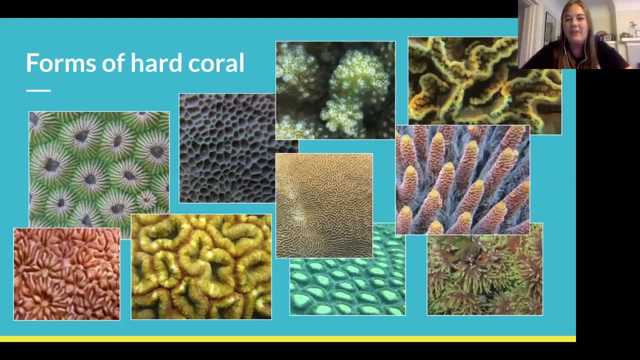 they want to feed, and most of the ones that you're seeing here have their tentacles retracted because it's daytime and so they wouldn't release their tentacles until later at night. but these structures at this very small scale provide, you know, a different sort of habitat for other species. 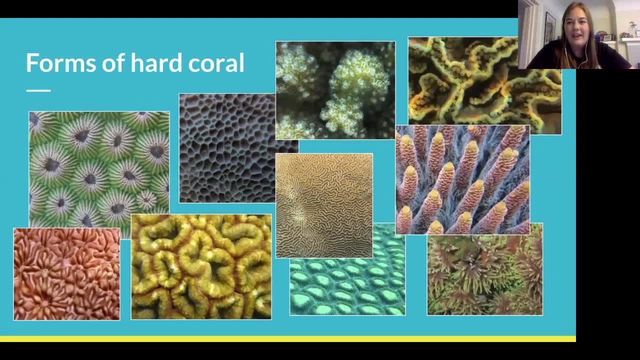 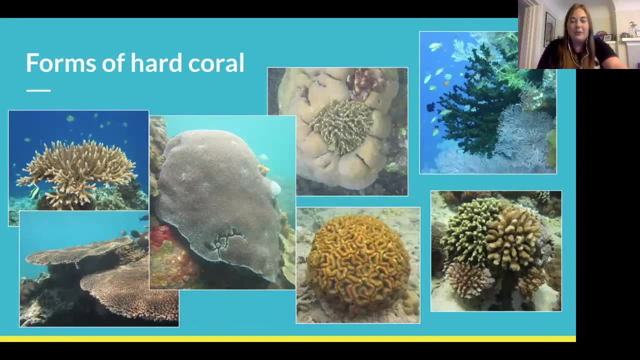 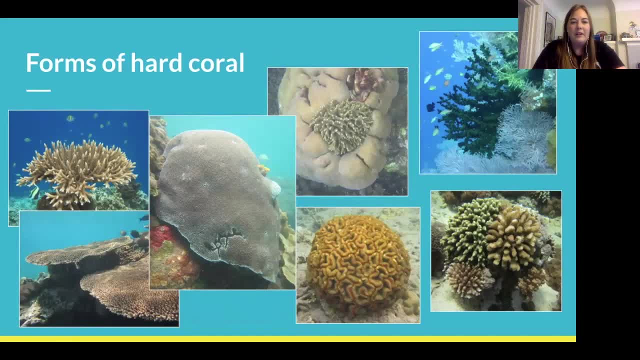 the one on the left here, or plating colonies, that's like make a flat surface encrusting colonies that we see in the middle here- massive colonies and then more different types of branching colonies, and so the branching corals really provide a lot of habitat for fish and other organisms to hide. the massive colonies also provide space to hide. 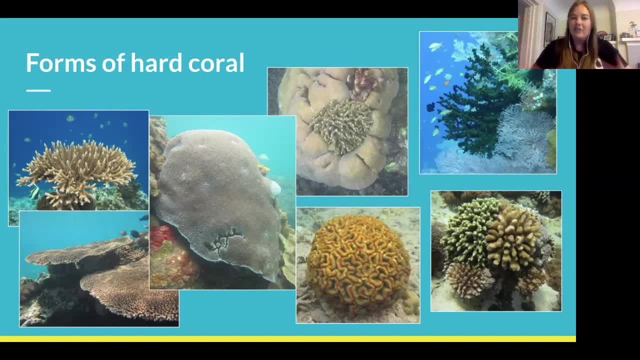 but you're more likely to find something under the massive colony than sort of you know there isn't a lot of nooks and crannies to tuck into um, and then you'll see that i mean these corals are growing literally on top of each other, and i'll get to that a little bit later. 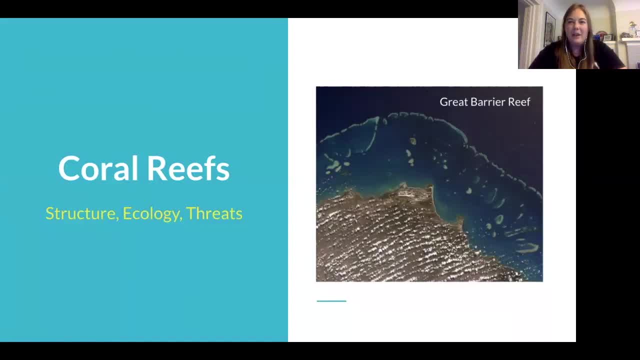 all right. so now we're going to scale up even more and talk about not just the coral polyps or the coral colonies, but the reefs that they create, from the structure to ecology, to the threats that they face, and these. so this photo shows the great barrier reef, which 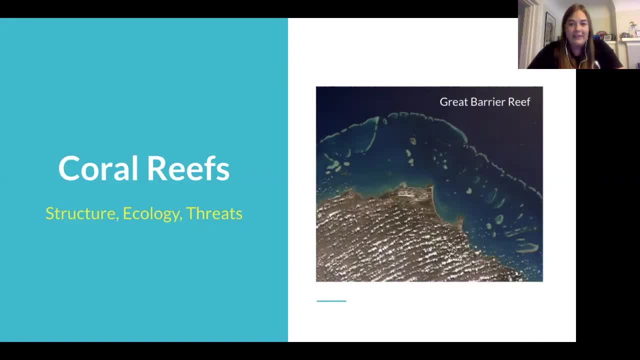 is the largest biological structure that you can see from space. it's very unique, but there are other barrier reefs around the world. this isn't the only one- and then there are a lot of reefs that are diverse, despite not being quite as big as the barrier reef, so we'll talk about that. 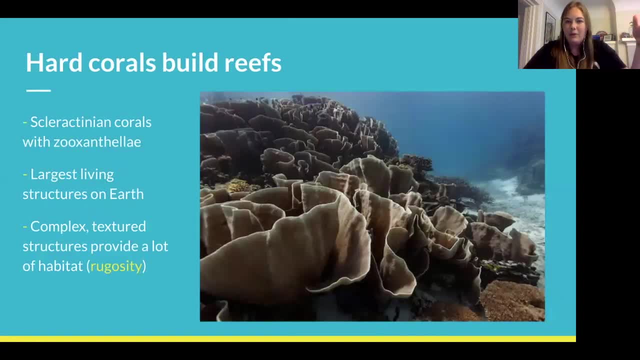 okay, so the i told you about those three types of corals, and it's really the hard corals, the sclerictinian corals with zooxanthellae, that build these huge structures. they are the largest living structures on earth and they provide this complex. 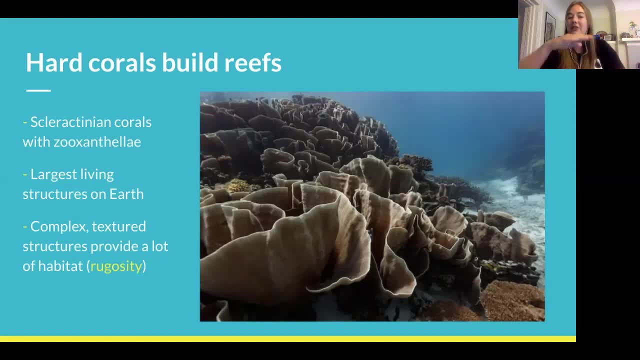 texture to habitat. and you can actually measure the texture of a coral reef, um using a measurement called rugosity, where you basically see, you know how how much, uh, what is the surface area of a certain reef, um in a certain physical area that you might think of? here's another, a different type of reef. 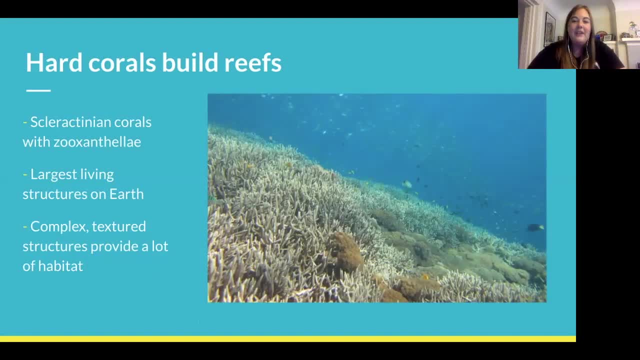 so the previous photo showed you a lettuce coral, this photo is showing you a croppera, and so you often do have these huge reefs that are all the same species of coral, um, that are providing and, and there there might be different species that live in association with those different. 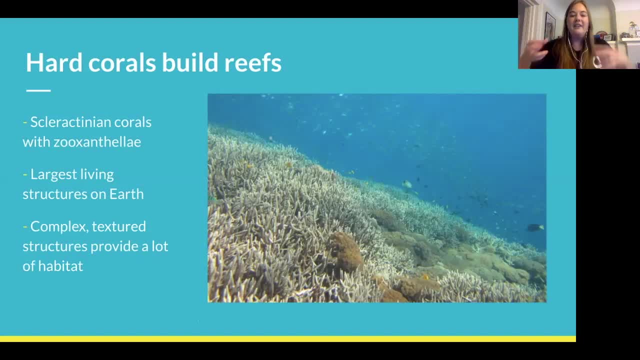 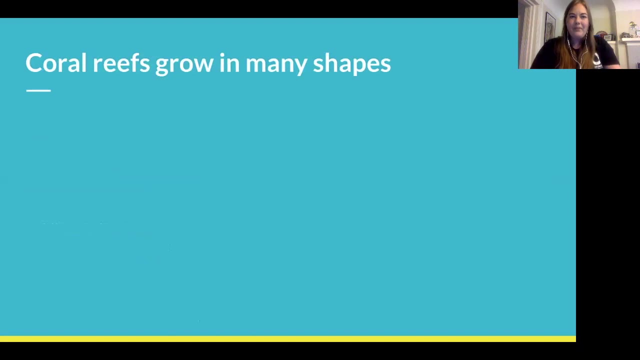 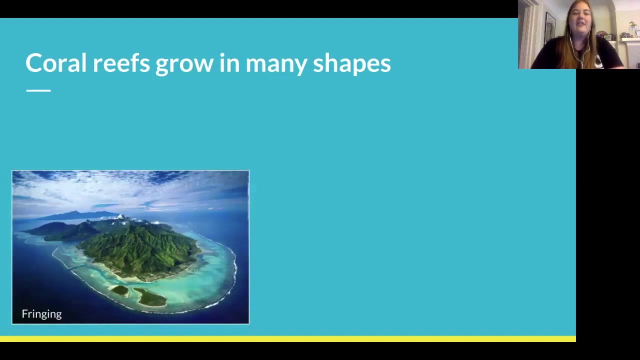 types of corals. so you see diversity in the, the whole community that is um living on these reefs. so, scaling up even further, we see that coral reefs form large, very large structures um and we've have different types that we've categorized these into. so fringing reef is one that's, you know, pretty. 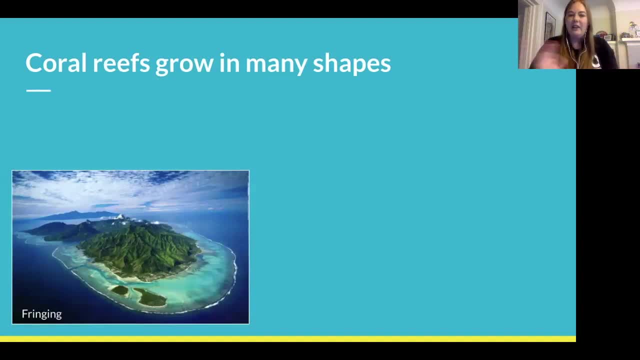 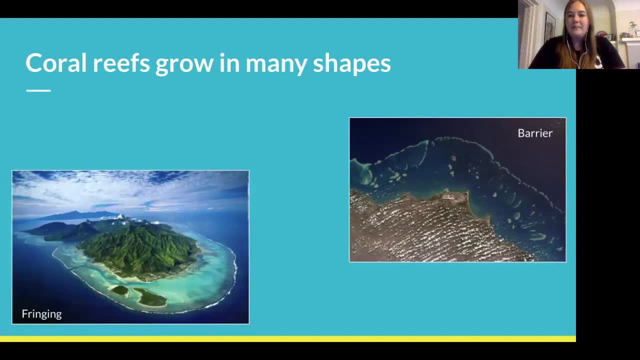 close to the land fringing around the land's edge. a barrier reef is farther out, away from the land and provides- uh, you know, both of these reef types provide protection from storm surge, waves etc. and then, within a barrier reef, you can have, um, you know, different types of structures as well. so 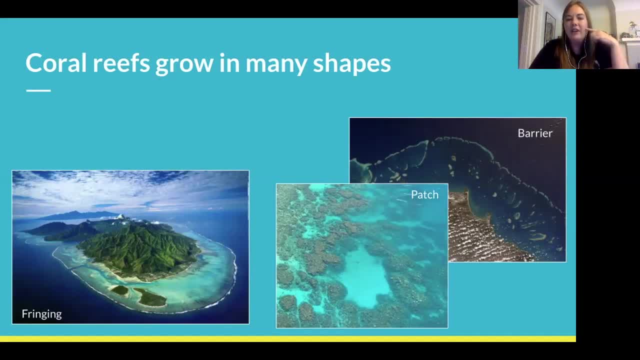 these. these next two are both actually photos from the great barrier reef. you've got patchy areas, usually kind of inside the edge of the barrier. you can also have ribbon reefs, which extend out away from the land for the coral reefs, and then you can also have reef types that are protected from the 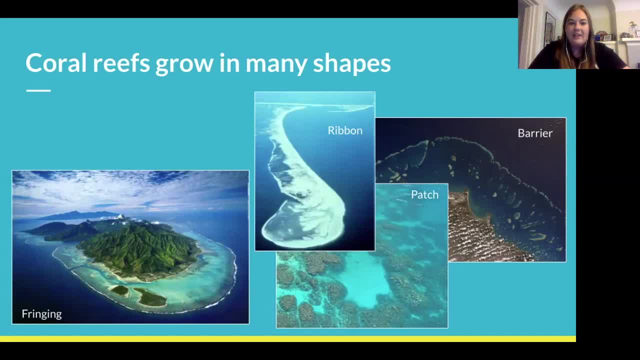 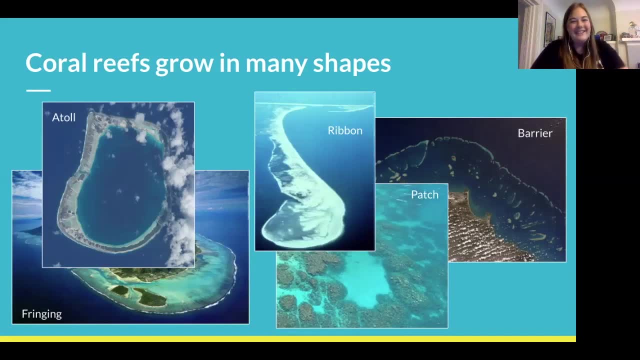 sand farther, and and then we also have what's called an atoll, where it's actually, you know, just the reef, without the island in the middle. and you may have learned about this in the geology lecture, but in case you didn't, um the way, the 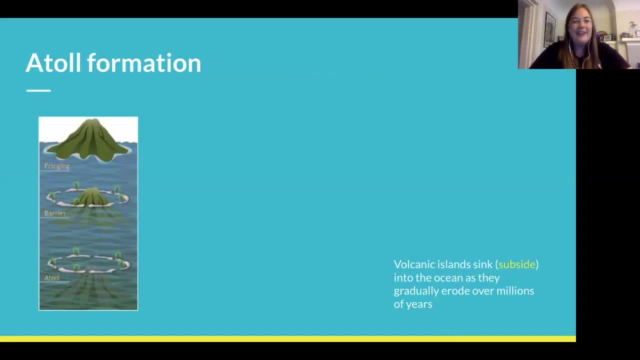 atolls. form is really cool and it has to do with the other reef types. so typically a volcanic island. you know it forms from underwater volcanoes. lava comes up, turns into land and island if it pokes up above the ocean, and so you get this: a reef growing around the outside of the island in the shallow. 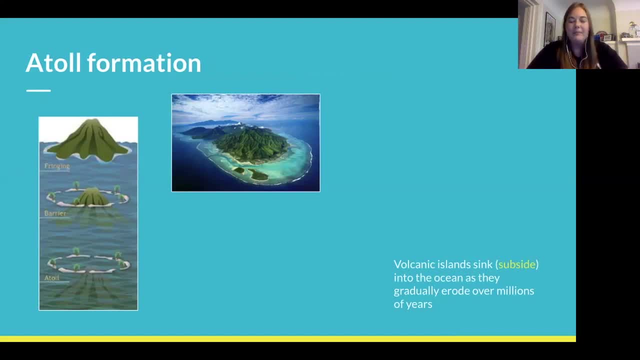 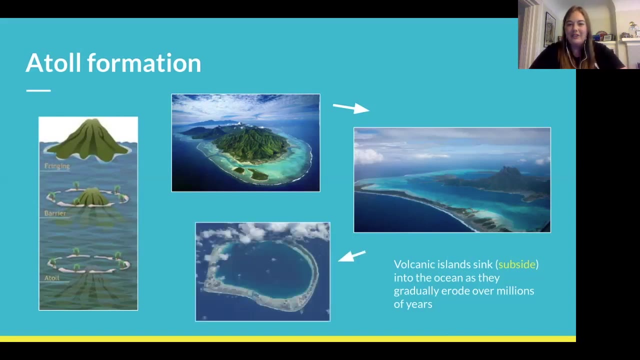 areas because reefs occur. large reefs grow where there's sunlight. over time the volcanic islands sink down or subside into the ocean because of erosion. this takes millions of years to grow and This takes millions of years, but eventually those islands can sink all the way down and leave just 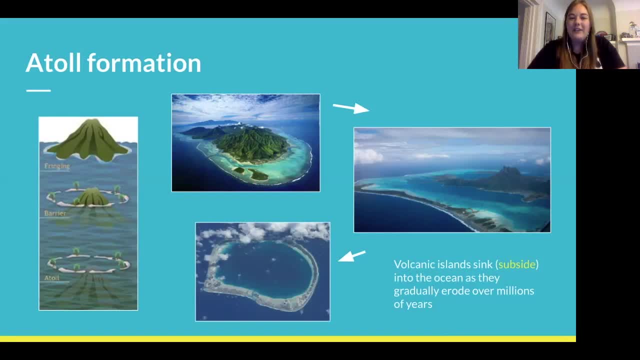 the reef behind, And the reef you know. you might say: oh well, why isn't the reef eroding as well? And it is. It's just that because the reef is alive, it's continuing to grow and if it can grow at the same rate or more than it erodes, it will stay there, even while the island. 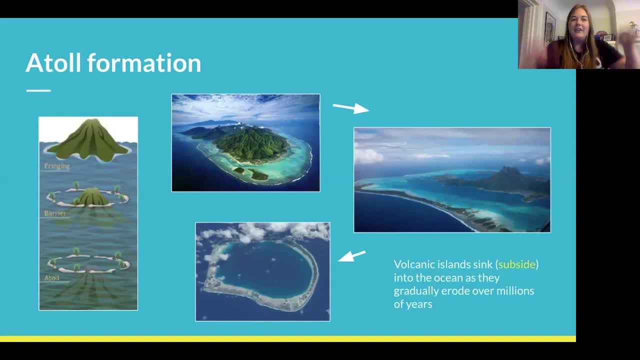 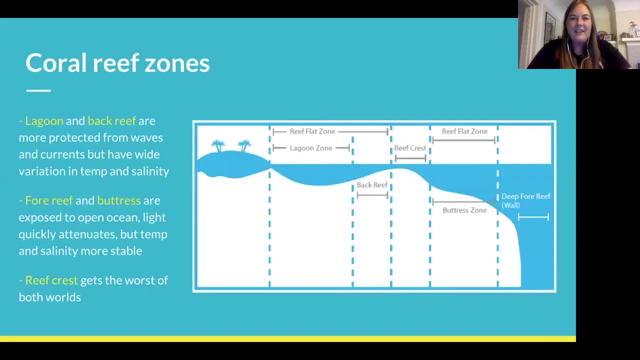 sinks, And so it's kind of like keeps growing up and up and up and I would love to. I would love to dive the middle of an atoll, but I never have. It's definitely on my bucket list, Okay. so, regardless of what type of reef you have, there's typically zones across that reef, and so 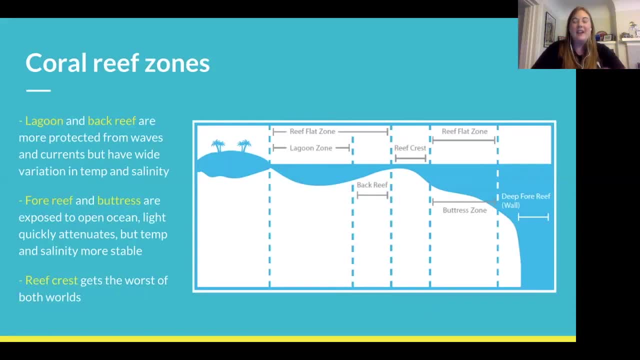 you know, one reef isn't going to have all the same habitat. There's going to be different types of habitats depending on what zone you're in, And the lagoon and the back reef are between the reef crest and whatever island is there, and so or continent, So that area is more protected. 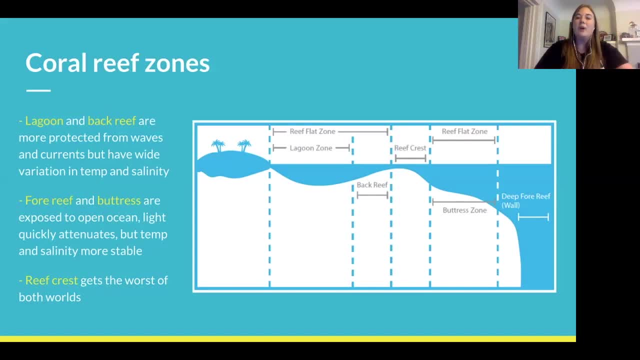 It's usually shallower, and so you can have water evaporating, causing some of the reef to sink, and so you can have all the same habitat. There's going to be different areas. There's going to be salinity to change. The temperature can change more easily because it's a 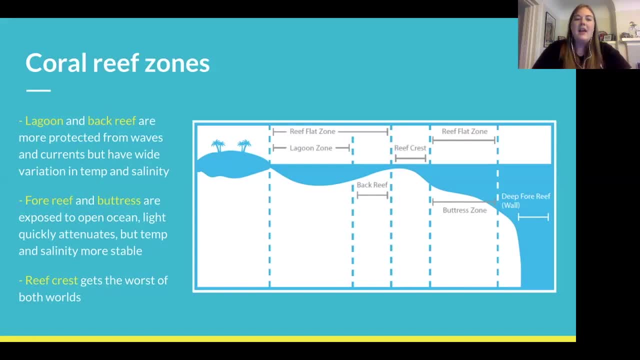 smaller, shallower body of water, And then, in contrast, the fore reef and the buttress zone are exposed to the open ocean, and so they're going to typically have colder temperatures, but not as much variation in temperature, And salinity will also be stable, because it's connected to the whole. 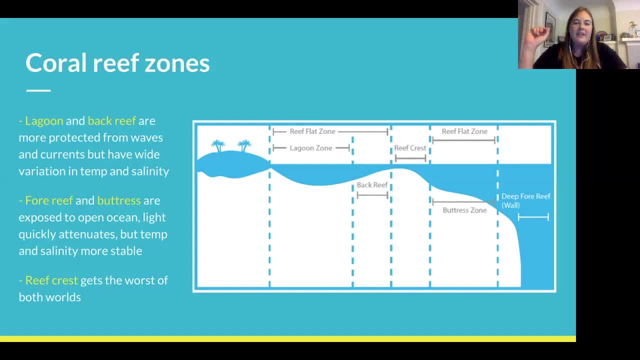 ocean And the wave activity and currents will be more prevalent and may cause, you know, struggles for whatever species are living there. And then the reef crest is basically the tallest part of the coral reef and it gets the worst of both worlds because it's shallow, so it gets, you know, really intense sunlight. It gets a lot of waves and 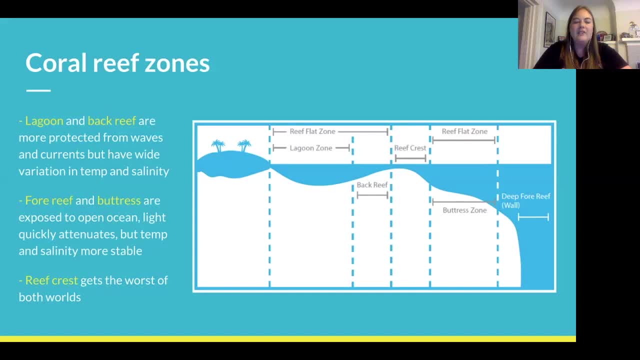 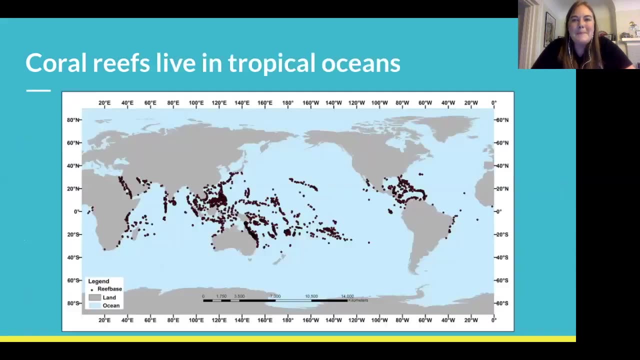 everything. So the reef crest is. there's not going to be as much living there, because it's a really difficult environment. Coral reefs do only occur in tropical oceans and you know this probably isn't news to you. This map shows where in the world coral reefs are found. 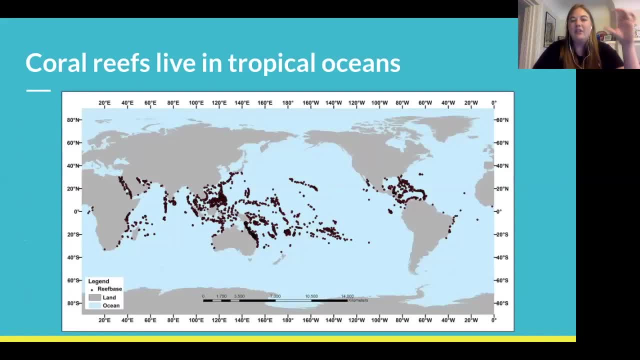 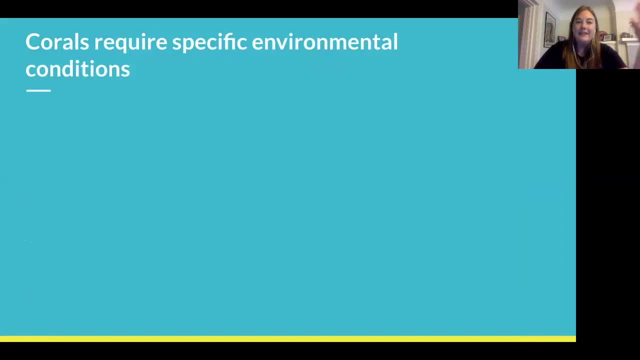 and it's really just between 30 degrees north and south for the most part. And why is that? It's because coral reefs require very specific environmental conditions. So, for example, if you have a coral reef and you have a coral reef, that's. 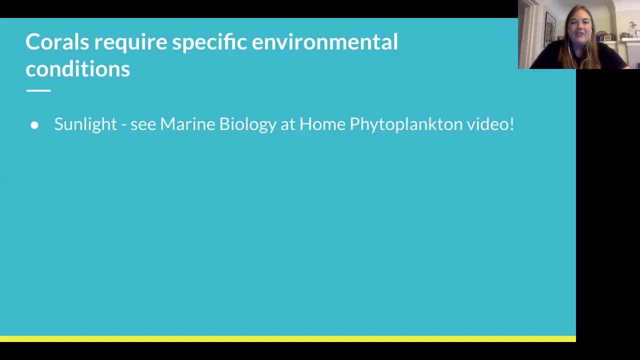 in the middle of the ocean, you can see that the coral reefs are in very difficult conditions, And the first of which is sunlight, And so if you want to know more about the- you know- distribution of sunlight around the planet and how that affects ocean life, I definitely. 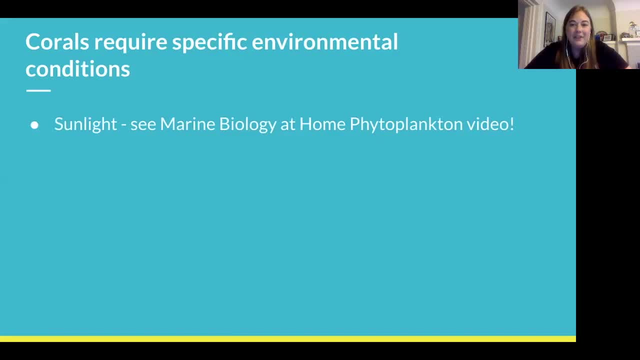 recommend watching the Marine Biology at Home phytoplankton video. Phytoplankton are doing photosynthesis, just like the zooxanthellae are that live in the corals, So they're going to have the same amount of sunlight around the planet, And so if you want to know more about the distribution of sunlight around the planet and how that affects ocean life, I definitely recommend watching the Marine Biology at Home phytoplankton video. 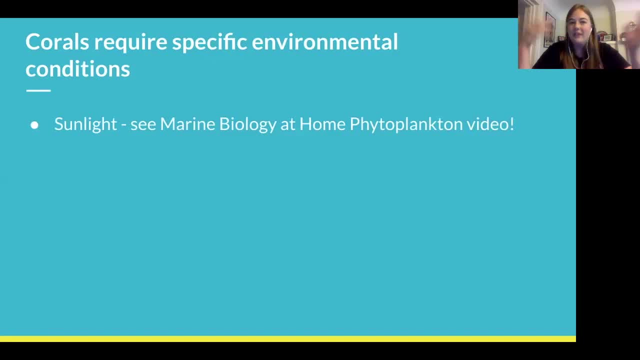 So if you want to know more about the distribution of sunlight around the planet, I definitely recommend watching the Marine Biology at Home: phytoplankton video requirements and sort of variety that phytoplankton have. Clear water is also important, And so clear water. 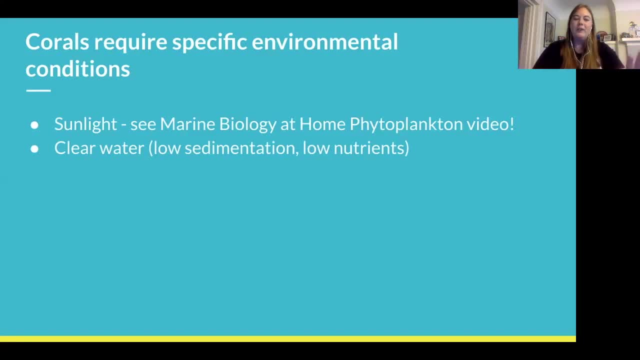 commercialού. There's two different things that affect water. One is sediment, which is basically, you know, Earth dirt that comes from the land out into the ocean, And so you want to have low sedimentation, fermentation, and then you also want to have low nutrients, because nutrients fuel phytoplankton. 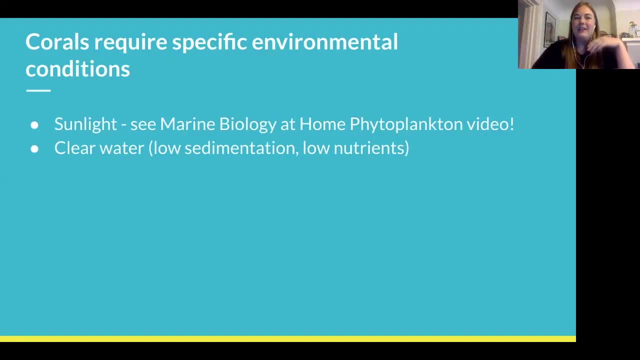 and the more phytoplankton you have in the water, the less clear the water will get. and so, yes, the phytoplankton, the corals, both like sunlight, but phytoplankton need nutrients, whereas the corals don't need as much. so, um, corals are going to thrive in areas where phytoplankton don't thrive. 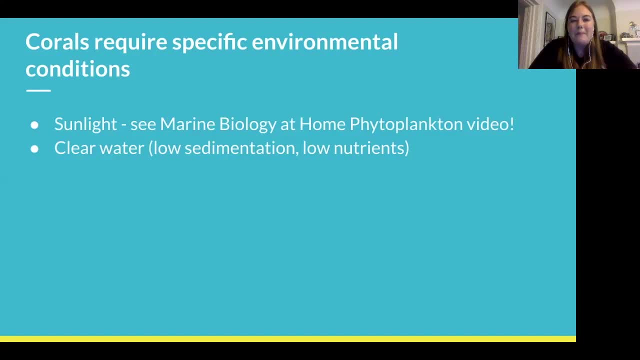 as much, and i know that's a little bit counterintuitive, because i was just saying that they both have similar sunlight requirements. but um, really it's that you know, corals and phytoplankton can coexist fine in an area where there's low nutrients, but in areas where there are high nutrients, the phytoplankton are going to do so well. 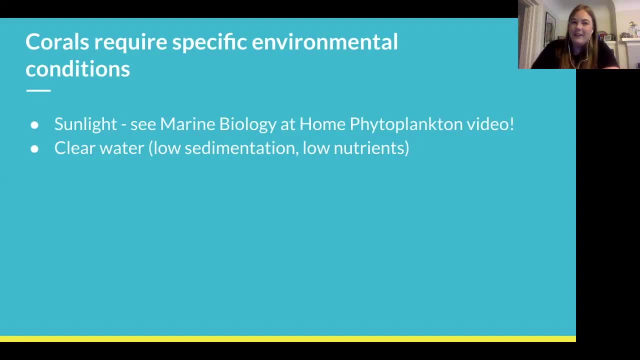 that the corals will not be able to get as much sunlight because it'll be blocked by the, by the plankton. hopefully that clarified it a bit. okay, warm temperature also important. corals have evolved in these tropical environments where there's a lot of sunlight, and so they're. 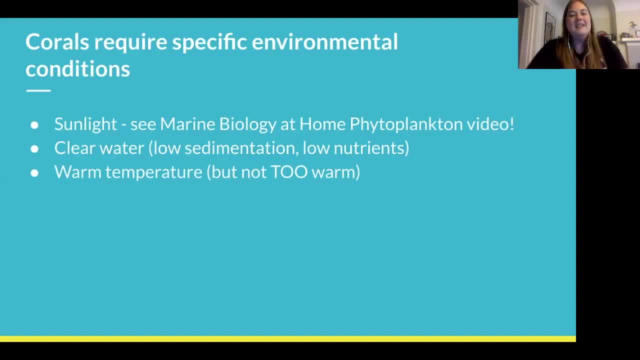 useless to the corals, and so they're not going to be able to get as much sunlight, and so they're not going to be able to get as much sunlight, and so they're not going to be able to get as much sunlight to warm water. But as we, you know, as you learned in the 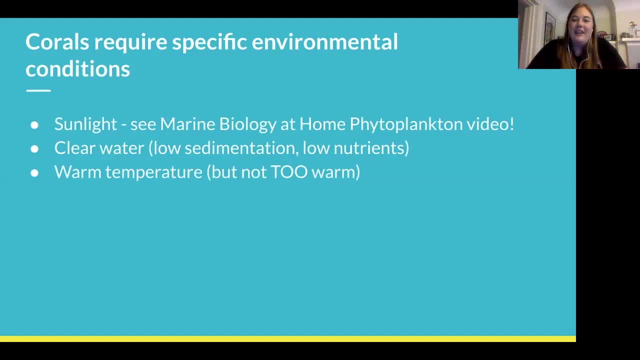 immerse video and which we'll talk a little bit more about later. if the water gets warmer than what they are used to in that area, they do get stressed out. They also need a hard substrate. So this is why corals only where coral reefs are. 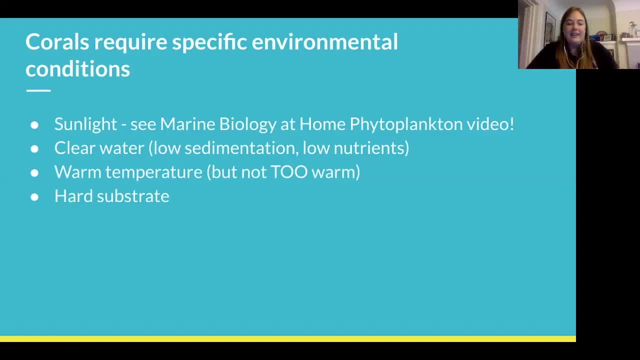 occurring in shallow areas. It's not just the sunlight, it's that they physically you know they have to be coastal shallow areas. you don't have free floating corals growing in the shallow ocean like open ocean right, they have to be attached. 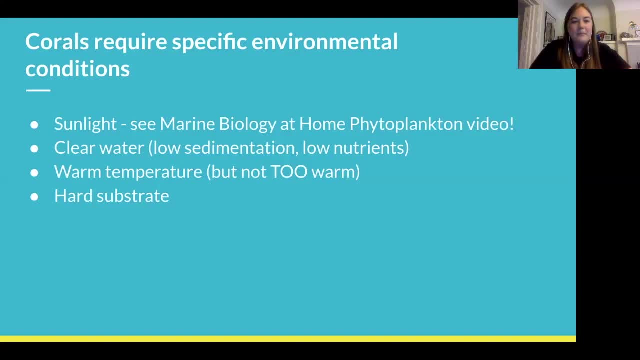 to a hard substrate. So they're coastal waters or around islands, And then they do have you know, usually have adapted to the local salinity conditions. So if you have a lot of fluctuations in salinity the corals will not be as well adapted to that. 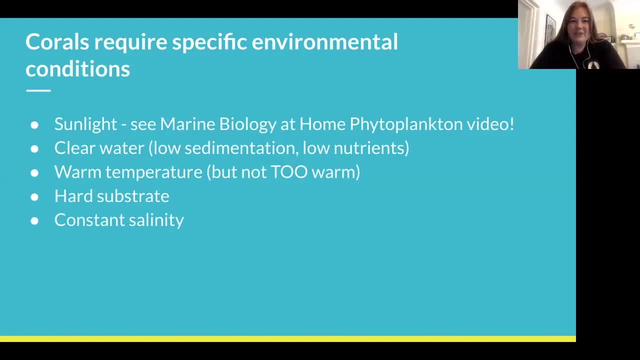 environment. So I was just editing this lecture video and realized I need to make a disclaimer about this slide. These are the conditions for hard reef building corals, because we're talking about the ecosystem of coral reefs And there are other corals that can live in deep waters without light, in cold. 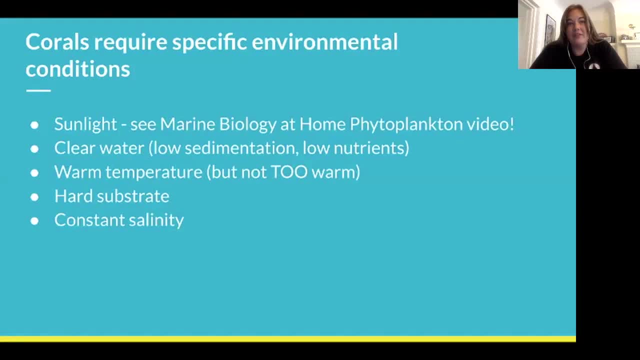 water, But they're just not the focus of this lecture. But I do encourage you to look up more about deep water corals and cold water corals, because they're they're very interesting. So one of the places that has all the right things for corals. 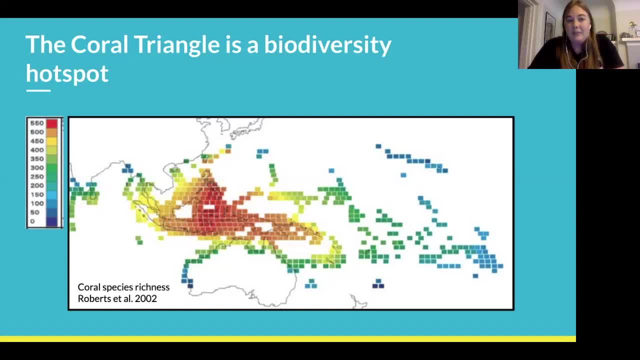 is called the coral triangle, And so we call it a biodiversity hotspot, And this is where Seabird and I met on a field trip, And it is defined by having over 500 species of coral, So any given wreath in this area. 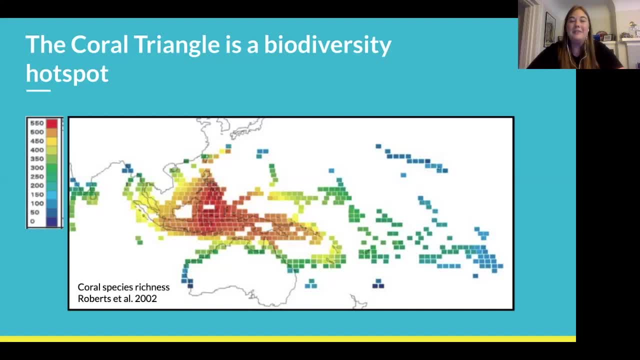 you might find 500 different species of coral, which is amazing. It's the highest species richness of corals of anywhere in the world, And so it's a really important area of study. I just wanted to highlight it because the Great Barrier Reef gets a lot of press- Rightfully, so. it's an 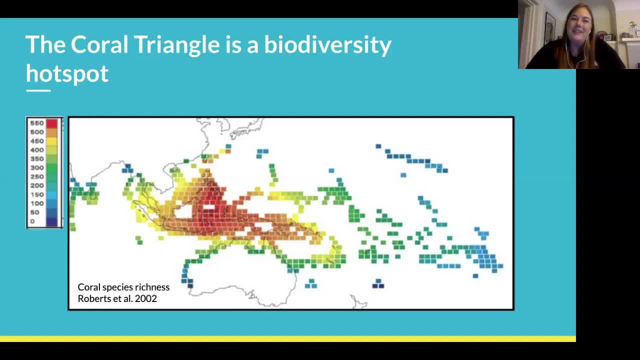 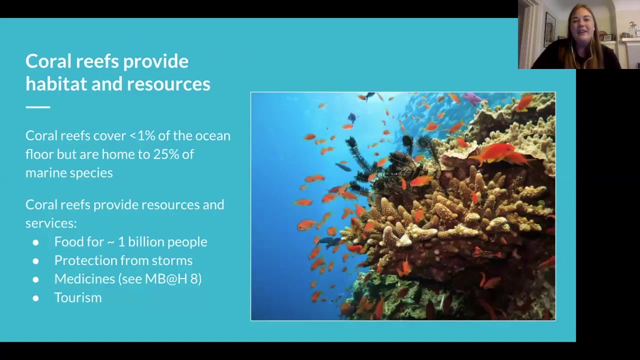 amazing place, But the coral triangle is a little bit less known, so I just wanted to put it on your radar as the place of the highest coral diversity in the world. And because there's higher coral diversity, you see higher diversity of other species as well, And that's because coral reefs provide habitat for other species. They only cover. 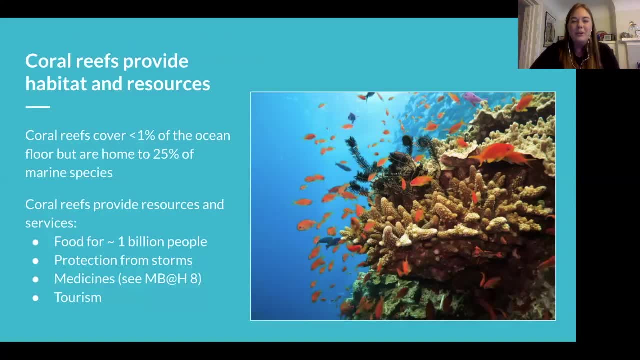 less than one percent of the ocean floor, but they're home to at least 25 percent of marine species, maybe even more. to be honest, This statistic gets thrown around a lot and I'm not sure the last time someone has checked. but you know, I wouldn't be surprised if it's actually more. 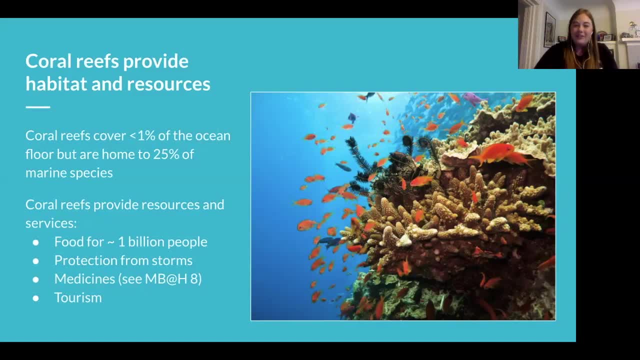 And coral reefs provide resources and services for for people as well. so it's not just about the other species they support. They also provide food for about a billion people. they provide protection from storms. just, you know, that's more than what they provide, but they also provide food for about a billion people. 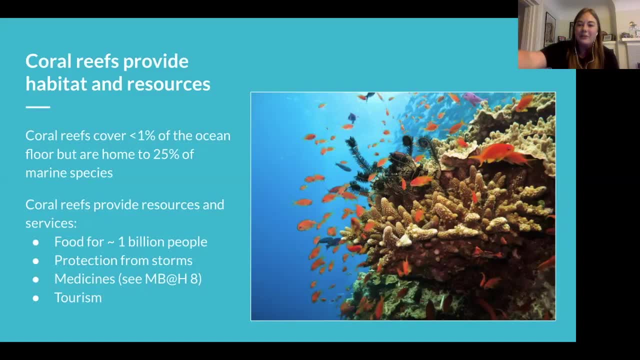 They provide protection from storms. just you know that's more than what they provide. One of the reasons that we have they're called barrier reefs. They're actually providing a barrier between the land and the open ocean, And storms as they're coming across that barrier will actually get weakened. 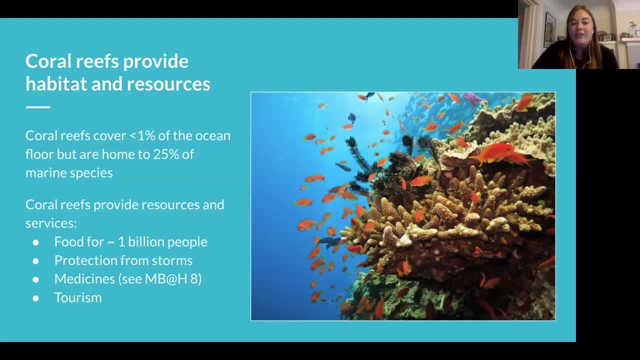 And if you watch the Marine Biology at Home- Lesson 8 on medicines marine- basically how we have been able to discover medicines using marine biology research- then you'll know about this already, But coral reefs are a rich source of some of those compounds that have been turned into medicines. 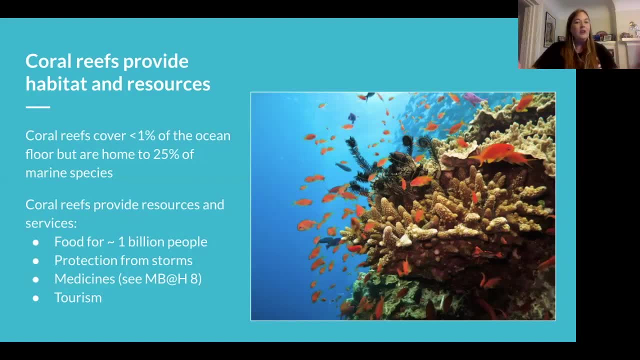 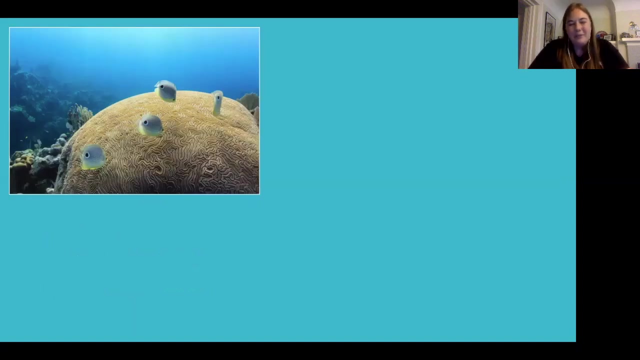 And they're also a great place for tourism, Which is a huge part of the economy of a lot of countries that are surrounded by coral reefs. So they're providing the- you know- livelihood for a lot of people in the world, Some of the. I just want to show you some of some cool photos from coral reefs now. 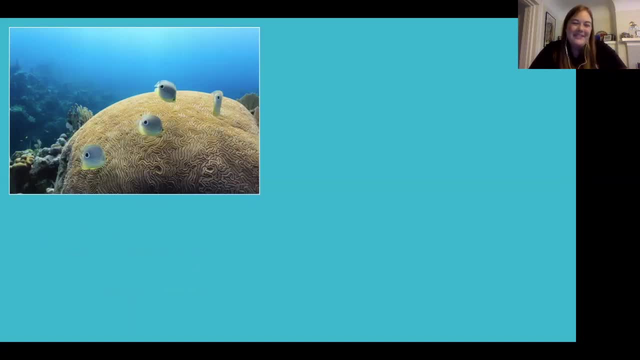 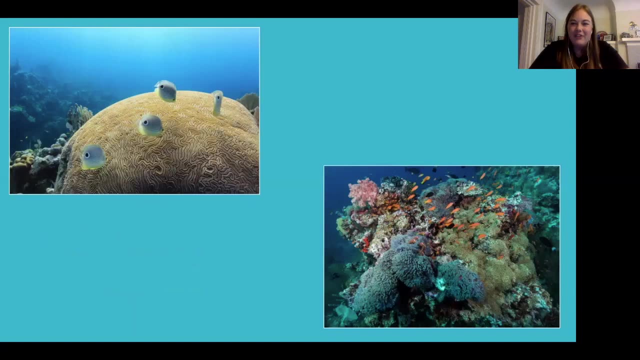 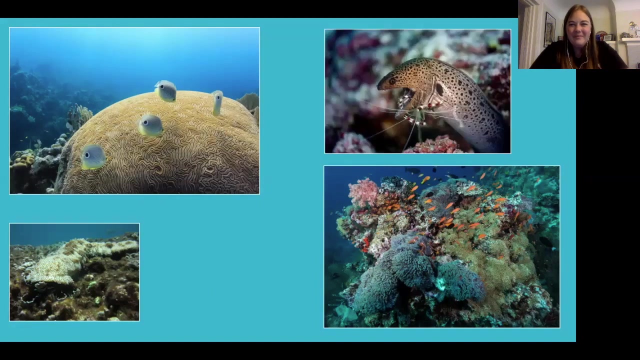 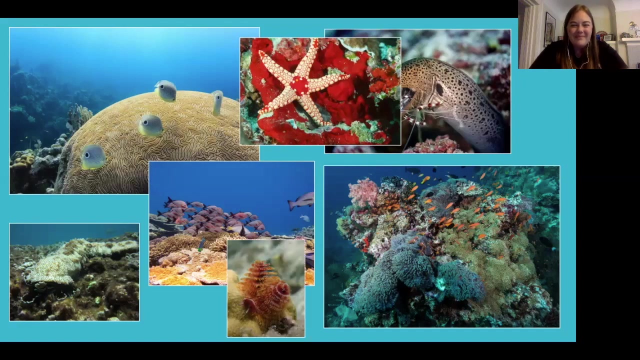 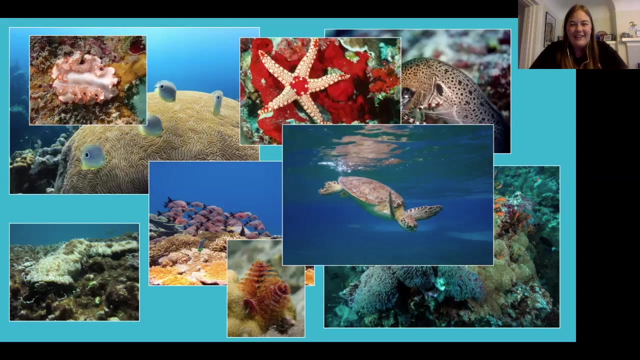 So we've got these amazing brain corals and fish. I showed you this photo earlier, but just like, let's just Let's just admire some of the diversity of species that live on coral reefs- And you know I talk a lot about invertebrates in my research, but you know we can't forget. 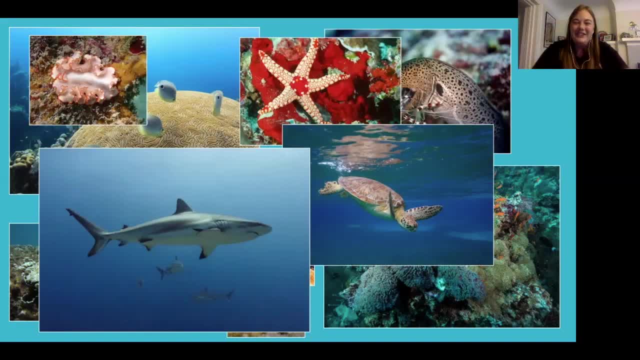 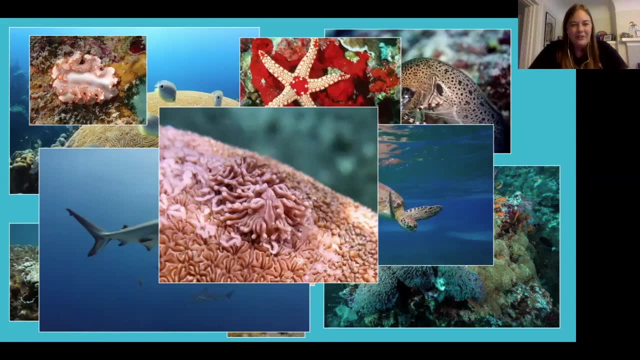 Everyone loves a good vertebrate as well, So sharks and sea turtles I'm always excited to see out there, And my favorite, the coral feeding nudibranchs. And I'm not going to tell you really about my own research, but I just wanted to show you that these nudibranchs are amazing because they're camouflaged on these corals that they live on. 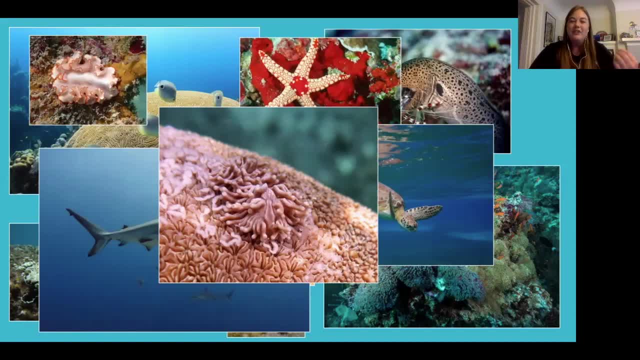 And so they've really adapted to live on a specific coral, and without the coral they just obviously would not exist. So I have corals to thank for these nudibranchs' existence, and I have Seabird McKeon, our course leader, to thank for introducing me to these nudibranchs. 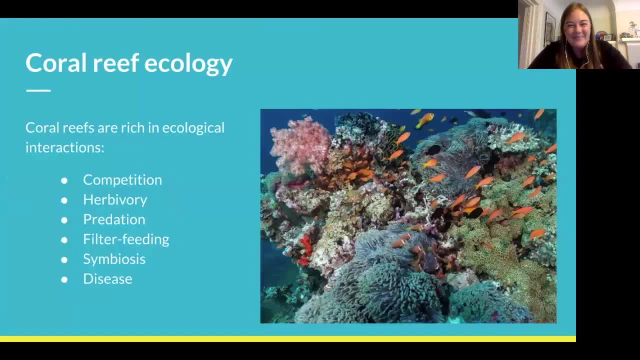 So thanks, Seabird. All right, so let's dive in- I'm going to use that a lot- to coral reef ecology. Coral reefs are rich in ecological interactions, just like any terrestrial ecosystem, And it's a pet peeve of us marine biologists when a general ecology course doesn't include marine examples, because 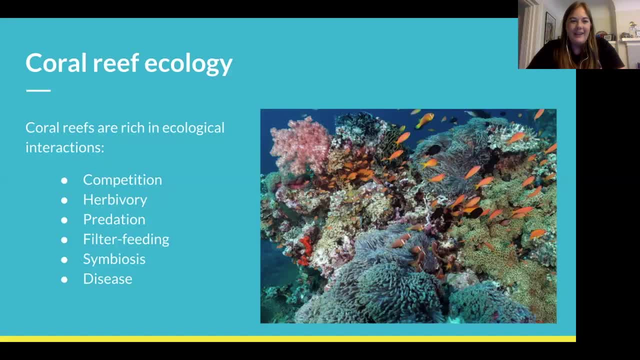 ecology is happening all over right. It's not only happening on land, And I do love that some universities and colleges have marine ecology courses specifically. but I still would would appreciate if more general ecology courses would incorporate marine systems into their coursework, because everyone should be exposed to this, these topics, And just because you know you're here so you're interested in marine biology. but I think if we talked more about marine biology in just general biology classes, then we could get more interest. 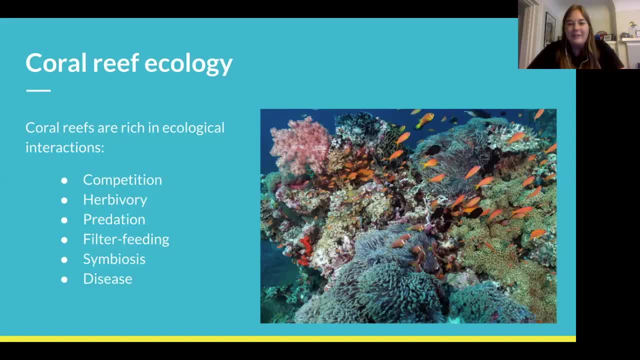 for the ocean and sort of garner, generate some of that ocean empathy that I would just love to see And everyone. So I'm going to go through some that you know, these different classic examples of ecological interactions and how they show up in coral reefs. 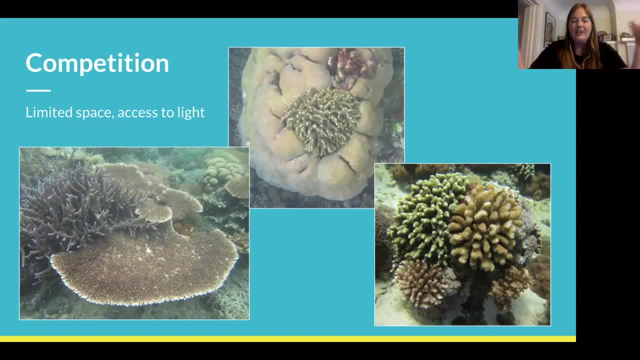 Corals and algae are always competing for space, So we've got these corals. you can see they're growing on top of each other Because hard structure, hard substrate is limited right and they need that, And they also need access to land. 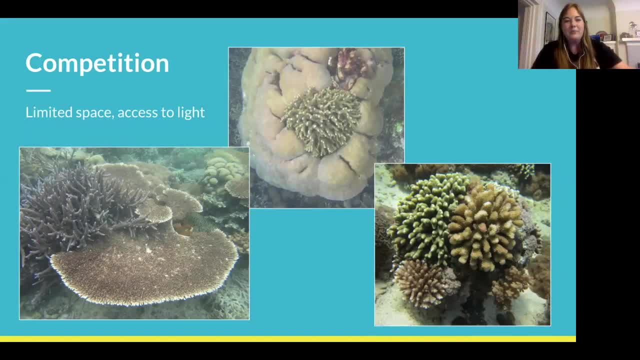 And so if something else is shading, you know this sort of expansive coral is shading out the area. this branching coral is kind of competing with that to break through and get the light and not be shaded right. So competing for light and space is big for corals. 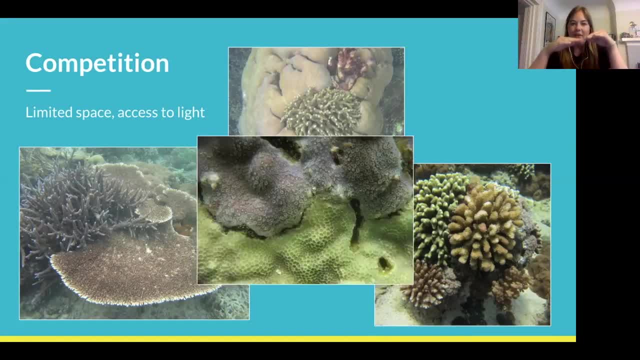 And also encrusting corals. you know they could so right where corals meet. if you look closely, they're kind of fighting a battle for space. So this photo- they've drawn their battle lines And this is just one snapshot in time. If I looked at this 10 years later, it might look different. right, The purple coral might have creeped in onto the yellow coral space a little bit. So they're always kind of battling each other at these boundaries. 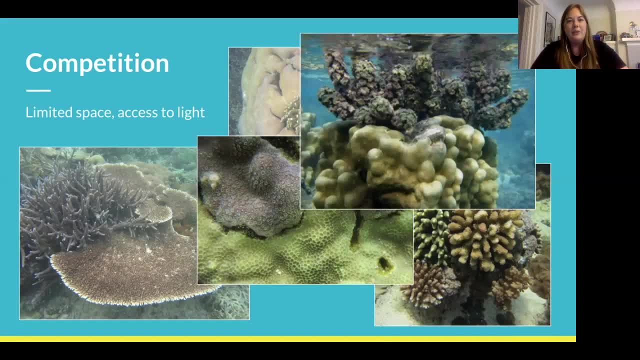 And they're also battling with algae. So this is showing a parites coral that has turbanaria macroalgae growing on top of it. That macroalgae is blocking the light of the coral And this is. there's a balance between macroalgae and corals in a healthy ecosystem, but sometimes disturbance will favor the algae. So, for example, the influx of nutrients, like I was talking about earlier. 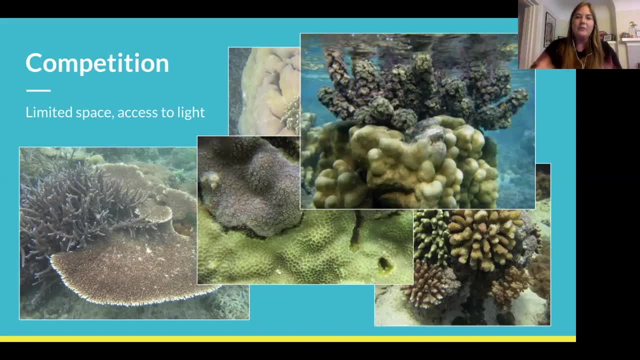 And so nothing beer entry there. So corals are still not goodoon for wyn 말고ia in general. So basically, you know, if this disagreement���standing, these two concepts of marine Bewegungen could basically spur some algae growth and they would block the light and the corals might die off and then you'd have an alcohol dominated ecosystem. 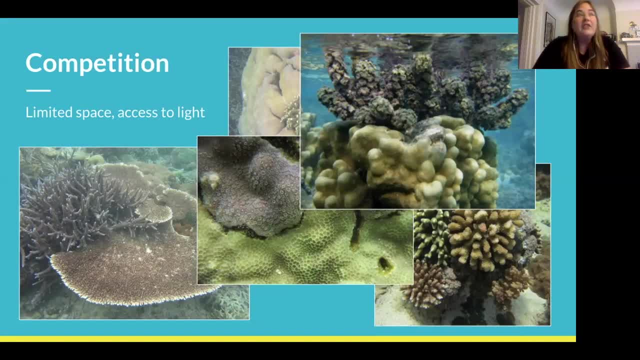 And there are certain species that do really well in that sort of ecosystem, But the diversity of coral reefs is still higher than these algae dominated systems. We kind of- I mean, I might be biased, but I prefer the coral-dominated systems personally- 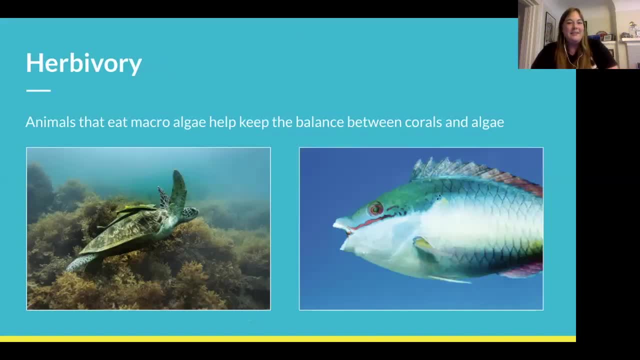 And luckily we have herbivores that help keep these macroalgae in check. So sea turtles are a great example and parrotfish another beautiful example of species that are herbivores and eat that algae and help the corals stay thriving. yeah, sort of ease. 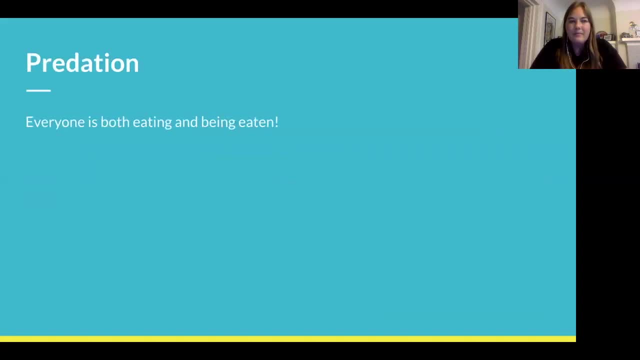 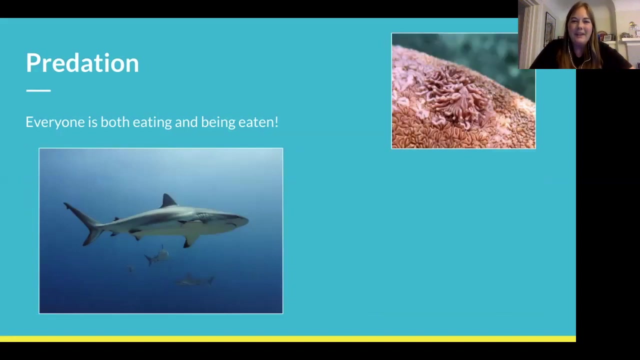 that competition a little bit, And there is a ton of predation on coral reefs, so everyone's either being eaten or eating something else, or both Sharks you may think of as the top predators. that's true, but something like the noodle. 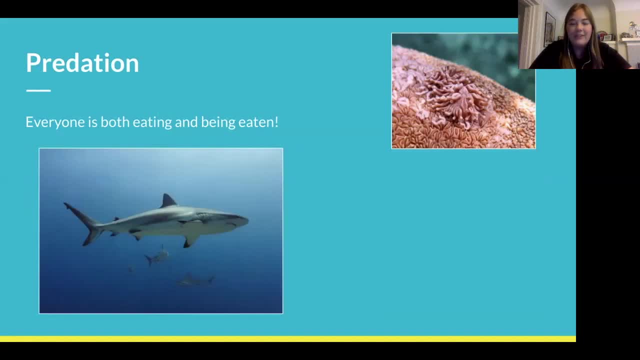 branks that I study are also predators. They're eating that coral. There's other noodle branks that eat. you know pretty much all noodle branks are carnivores. They're eating some sort of other invertebrate like sponges, hydroids, sea anemones, whatever. 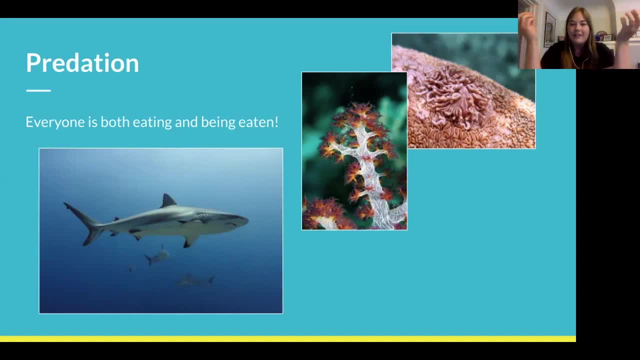 Corals themselves are a predator, right, I was talking about how the tentacles are stinging and capturing plankton out of the water. That's a predator. That's a predator right there. Corals are predators. And then we've got fish that eat corals. 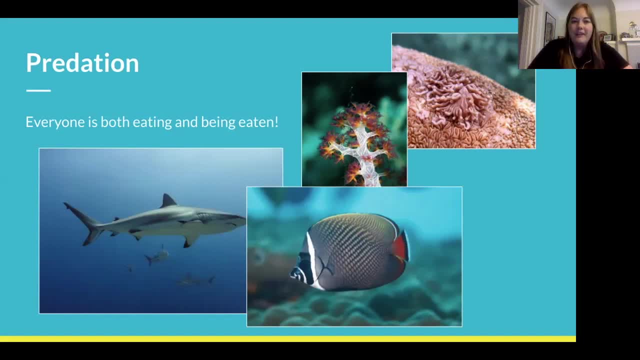 So you know, corals are a predator, but they're also being eaten, right? There's really really multi-level, complex food webs on coral reefs And then we've got- yeah, so more fish that are actually eating coral polyps- also fish. 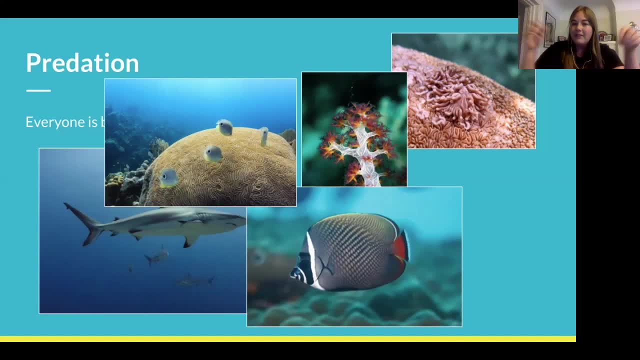 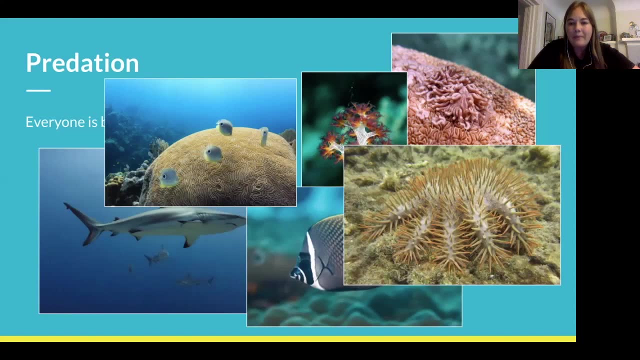 that are eating, You know, tiny invertebrates off of the corals, which I think is what these butterfly fish are doing. And then we've got the meanest of them all, acanthaster, which is the crown of thorns starfish. 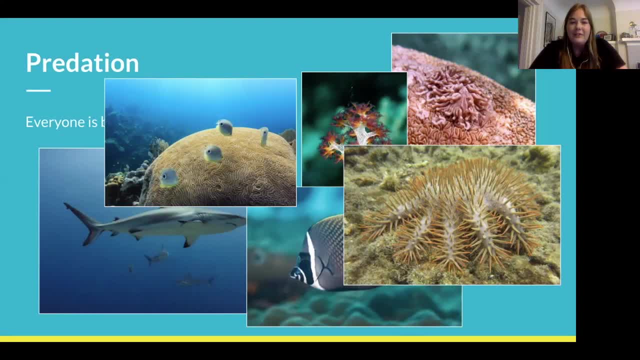 And so this is a coral predator that is voracious and has actually caused a lot of problems. Because if a coral reef isn't doing that well and if the coral reef isn't doing that well, and if the coral reef isn't doing that well and if the coral reef isn't doing that well, 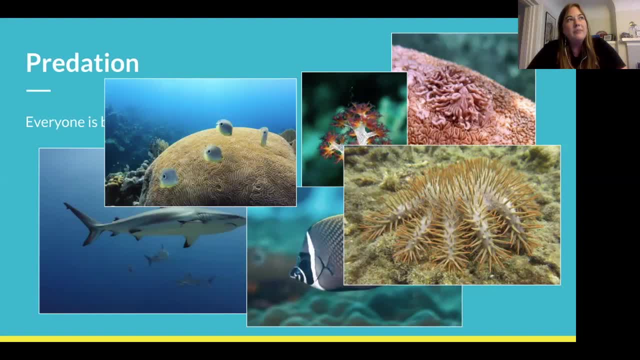 the. you know there are some, um some kind of larger animals, actually don't know what, eats acanthaster, but if the predators of acanthaster aren't present present, then they can bloom and basically destroy an entire reef by eating the coral, And so this has happened in French. 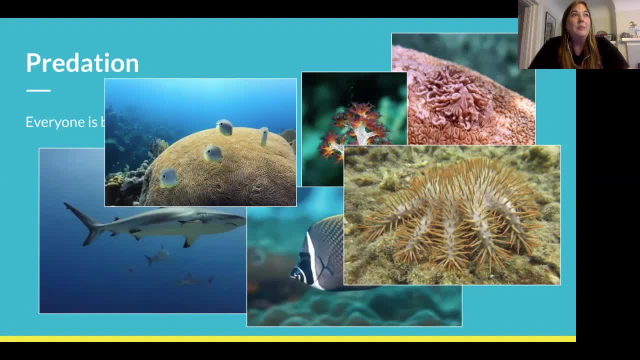 Polynesia and um, it is a problem. Um, it's something that we as humans can kind of intervene in. If we see it happening, you know, we can capture them and stop it, But um, unfortunately it's kind of just sort of natural uh predator that's out there. That's a big threat for corals. 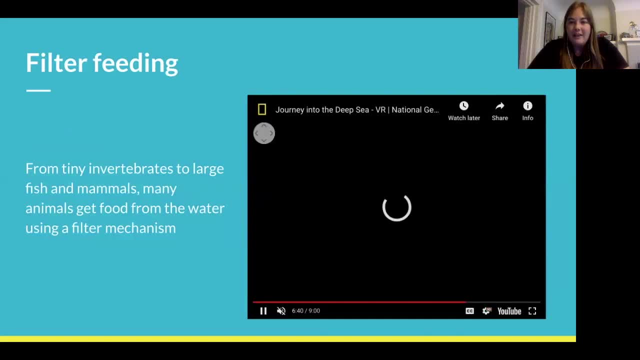 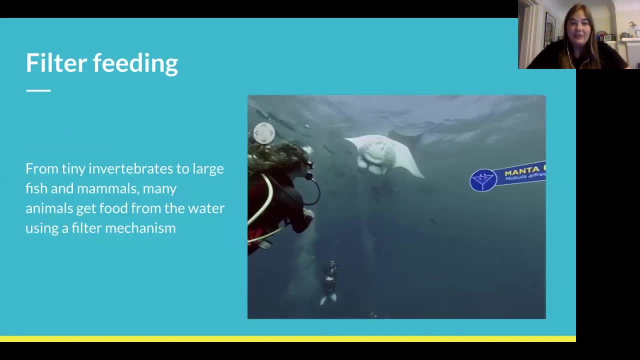 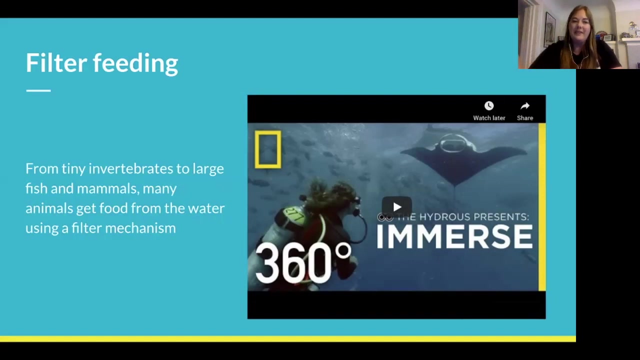 So filter feeding is a really common um marine way of life, something that you don't see in terrestrial environments. So things um from you know, tiny invertebrates up to big reef, manta rays like you saw in Immerse. use a filtering mechanism to get plankton out of the water. 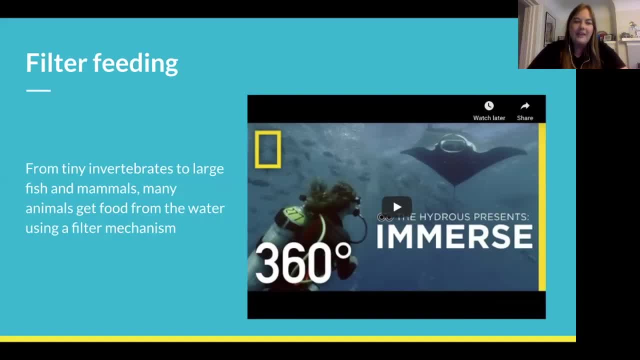 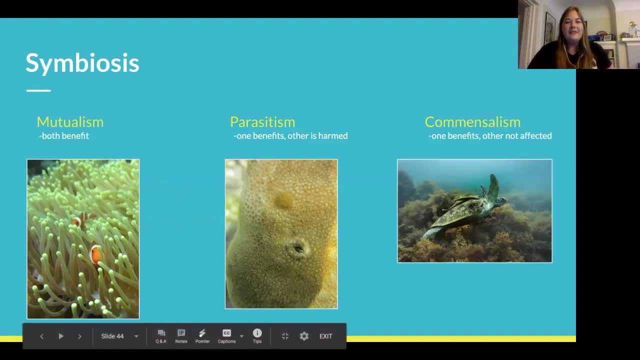 So just wanted to include that as something that's kind of unique to the ocean. Now let's get into symbiosis. So I already talked about mutualisms. I gave you that example of the zooxanthellae living in coral reefs, And we also have our classic example of anemone fish and 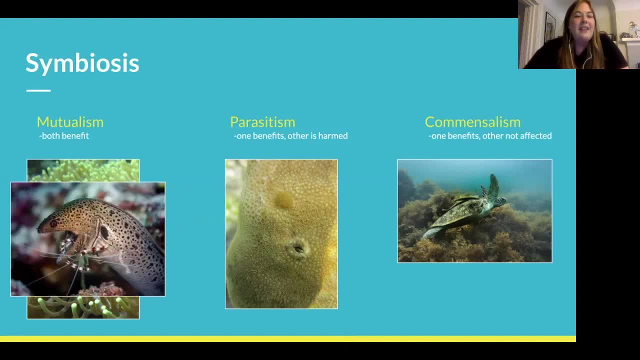 anemones, But another one that I love is these cleaner shrimp, And so they're basically the dentists of the reef. They will eat um anemones and they will eat um anemones, And so they'll. 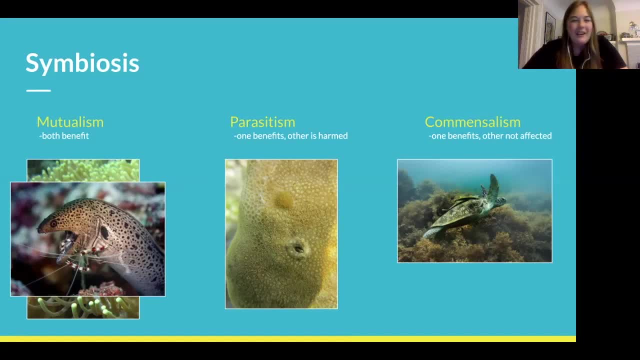 Little particles, sort of dead items and whatnot, out of the teeth of fish, like this eel here, And so you know the eel gets a great cleaning out of it. right Got to keep your teeth clean for optimal health. 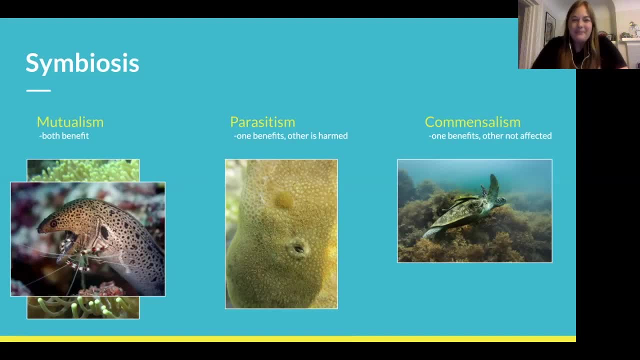 And the shrimp gets food out of it. So it's a win-win And they're very cute. And then we've got parasites. So here I'm showing you a coral that has- it actually has a nudibranch on it. So that bump, the upper bump, is, yeah, right in the- you know, the upper half of the photo. 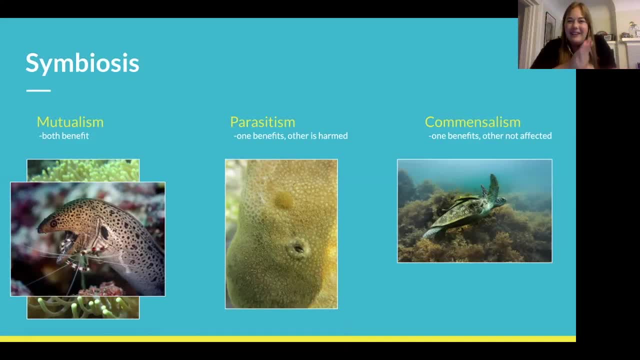 That's a nudibranch that is attached to the coral and is eating coral polyps. It's some people call these predators. I think this species, Pinupeus rebus, should be categorized as a parasite because of its- you know- attachment to the coral. 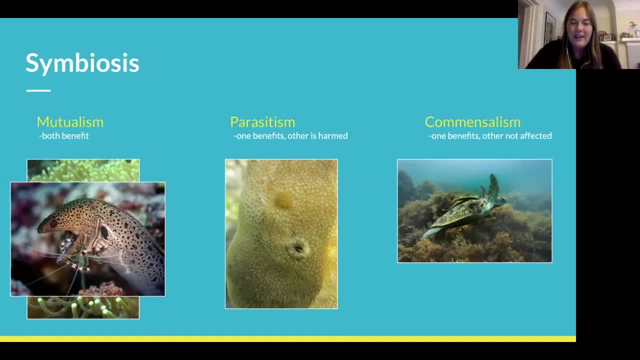 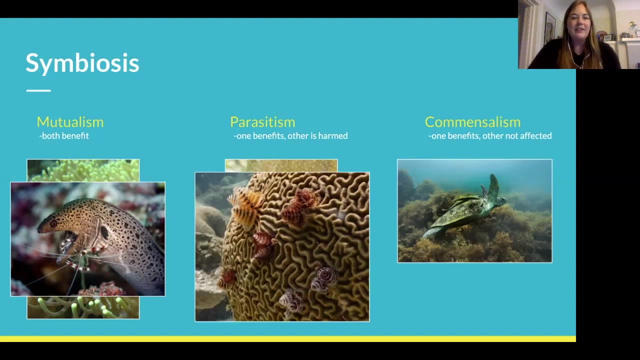 And then below that there's a boring clam, So that little hole. there's actually a clam that has bored into the coral and is living in there and like peeking out a little bit. And another invertebrate that bores into corals are these Christmas tree worms, which are so cute and beautiful. 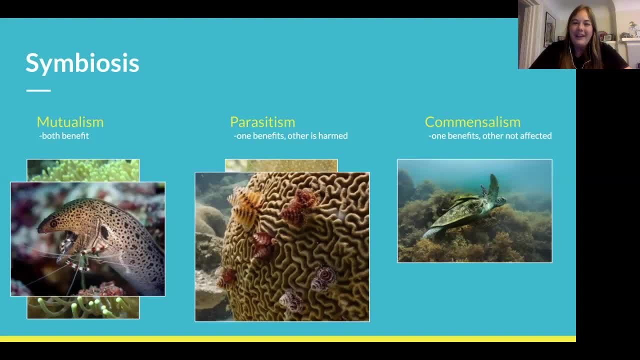 They're really colorful. But you know they have taken, they're taking something away from the coral by, by, you know, taking something away from the coral boring into its skeleton right, And they're blocking sunlight from those areas. So they're. 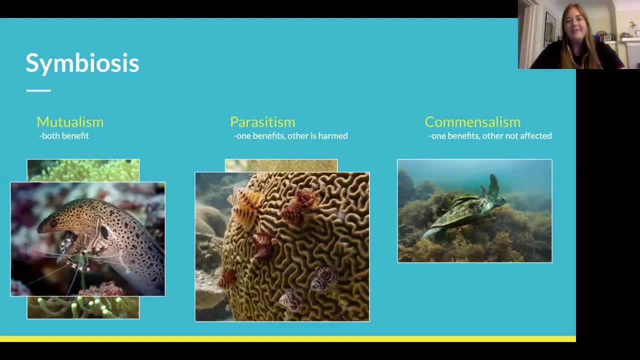 harming the coral for their own benefit, but the coral is actually doing fine. So it's, you know, a little bit of harm, but not so much that it kills the coral. And then commensalism, which is when one benefits and the other is supposedly not affected. The kind of classic example is these: 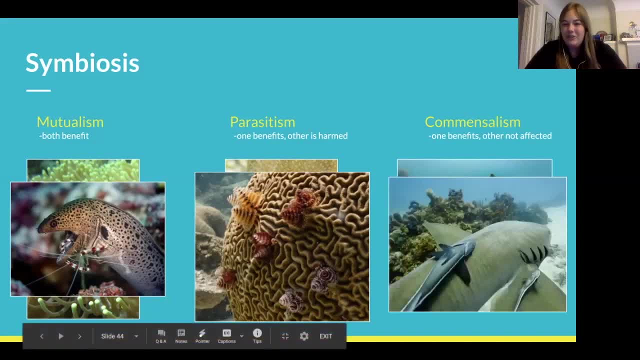 remora fish, which will attach to sea turtles and sharks and hitch a ride. You know, they say that the turtles and the sharks are not really affected by this. I feel like there must be. there may be a slight effect when it comes to the fluid dynamics of moving through the water, but 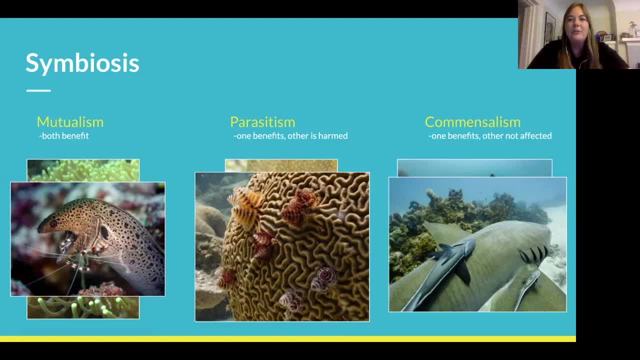 it's. I guess it's inconsequential. So we consider this a commensalism And I'd love to hear other examples that that you can think of of each of these. So on the Facebook group, you know we should start a thread for symbioses on the in the reef, because they're 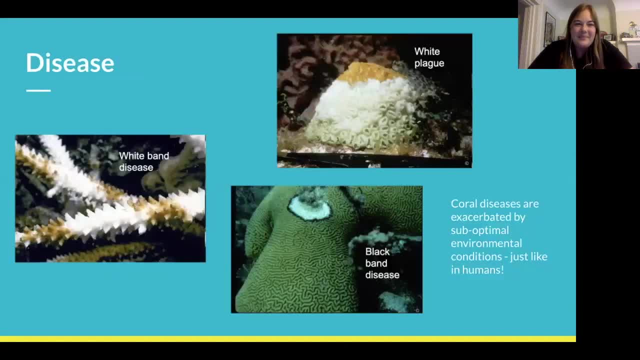 one of my favorite topics. All right. next we've got disease. So diseases do occur naturally on coral reefs. I'm showing a few examples here, And you know, just like human diseases, there are factors that can make them either better or worse. 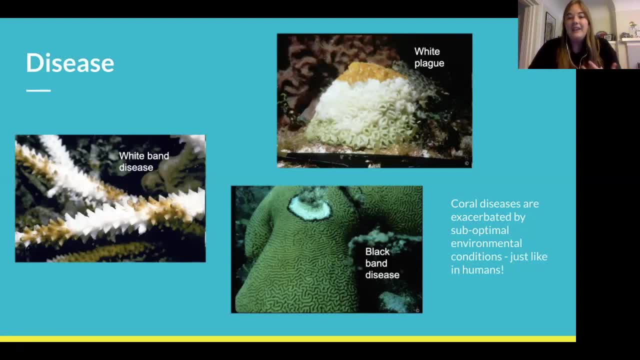 And the environmental conditions that you're in can have a big impact on the immune response to a disease, And so I'll use COVID-19 as an example right now. If you have a preexisting condition or some sort of environmental factor like- perhaps you know- asthma, which can be- you know, asthma is. 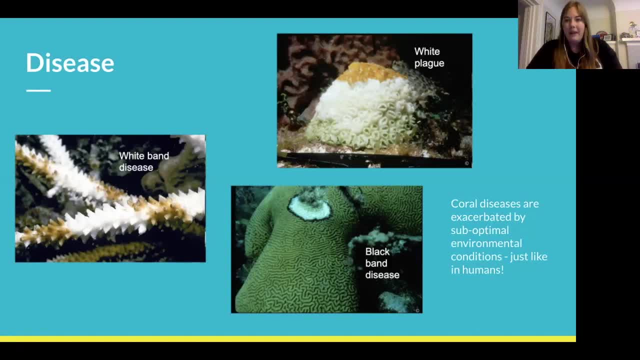 something that is exacerbated by the environment. And then if you add a respiratory disease like COVID-19,, the combined effect is going to be very harmful. Similarly with corals. you have diseases which the corals are naturally fighting with their own. 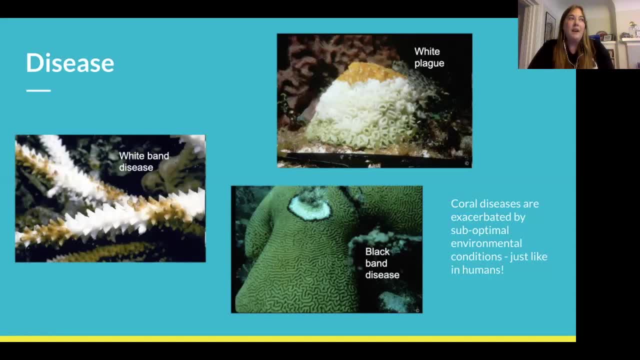 immune response, But if the coral is stressed by higher temperatures or pollution, the coral is more likely to lose the battle against the disease. So this is something that we need to think a lot about, especially with climate change, which I'm going to get to a little bit later. But disease is a natural ecological process. 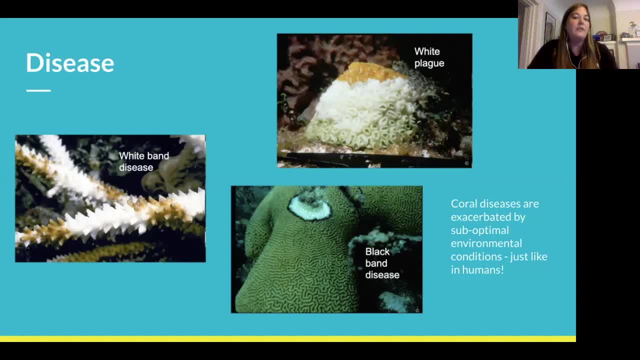 You know it's an interaction between microorganisms and corals. So I'm not going, I can't, we can't attribute it solely to human intervention. It's just part of the ecology of coral reefs, But humans can definitely make it worse. 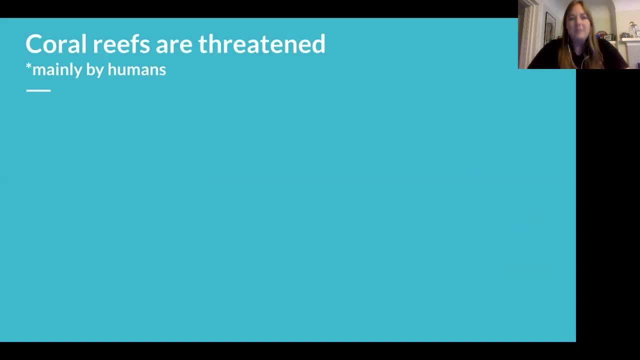 All right. so here's some of the other ways that coral reefs are threatened, mainly by humans. We've got coastal development, coastal runoff, which contributes to sedimentation and nutrient pollution. So those are things that affect the water clarity that I talked about earlier. 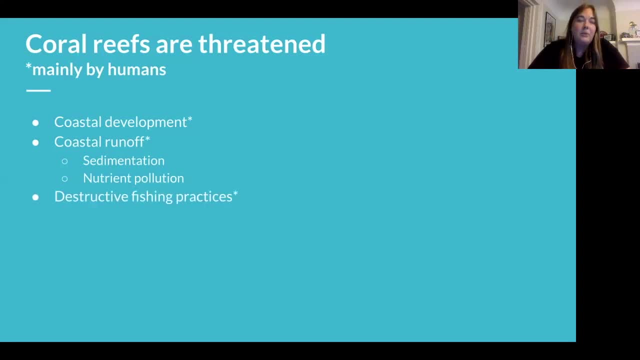 And destructive fishing practices. So fishing is an important part of human life. I'll talk a little bit more about this later, but there are ways to do it that are safe for coral and there are ways that are not so safe. Plastic and other trash are a big problem for reefs as well. 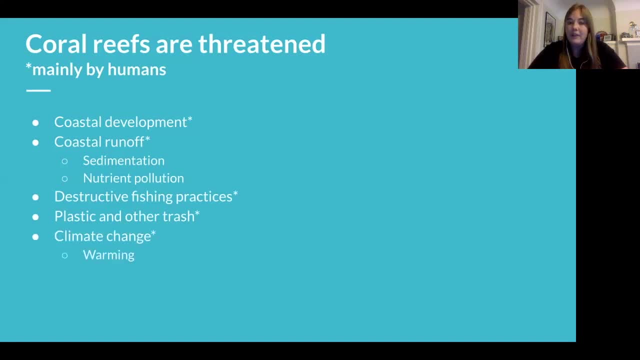 And then climate change- big one, especially with warming of oceans and increased storm activity which damage any coastal environment, right? So we just had a hurricane come through. You know you could be watching this anytime, but I am making this lecture the day after Hurricane Laura hit the United States. 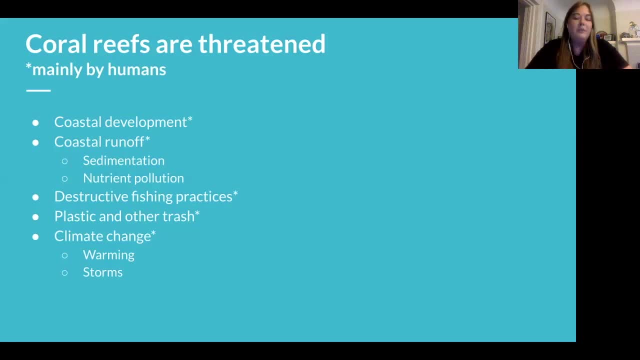 And so you know, the Prevalence of storms and the strength of storms is going to be affected by climate change, and corals are a great barrier because they take the initial brunt of storms, but if they're damaged by the storms, then they're not going to be able to protect us from the next storms, right? 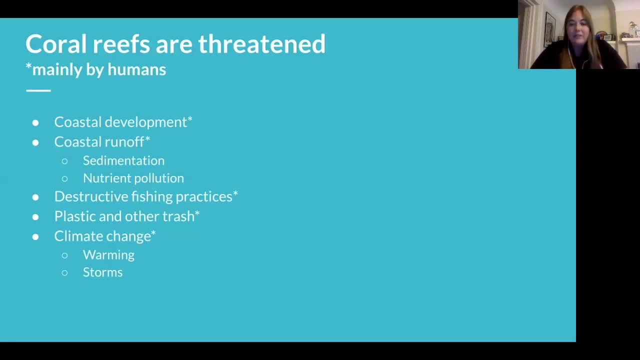 And that's bad for us and it's bad for the corals. And then we also have ocean acidification, Which I'm not going to go into much detail about, But I highly recommend you Do some additional research on this if you want, but I think it might be covered in some of the other the other lecture topics as well. 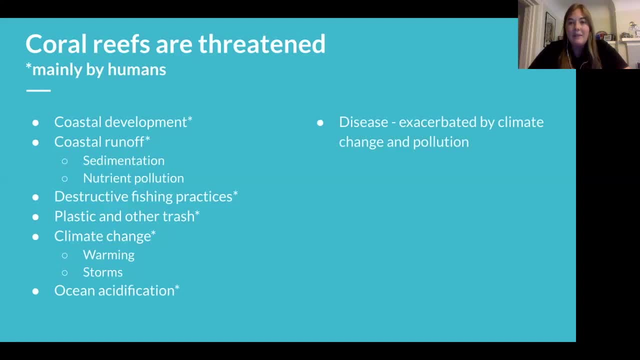 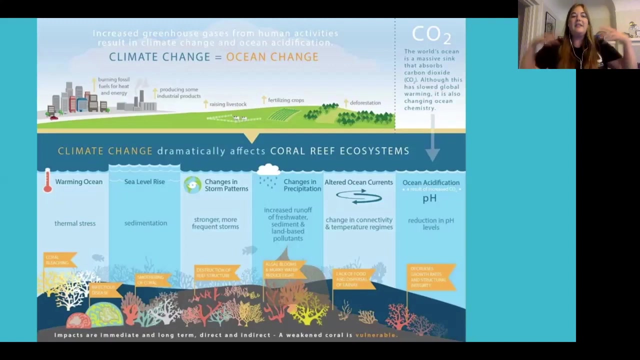 And then I've already talked about disease and how that's exacerbated by climate change and pollution, and then the chronophore and starfish, which are also a big threat to corals. So I want to Focus a little bit on climate change, because it's the biggest threat right now to coral reefs and it's caused by increasing carbon dioxide in the atmosphere, which comes from burning fossil fuels and raising livestock and also is exacerbated by by deforestation. So, as carbon dioxide is, 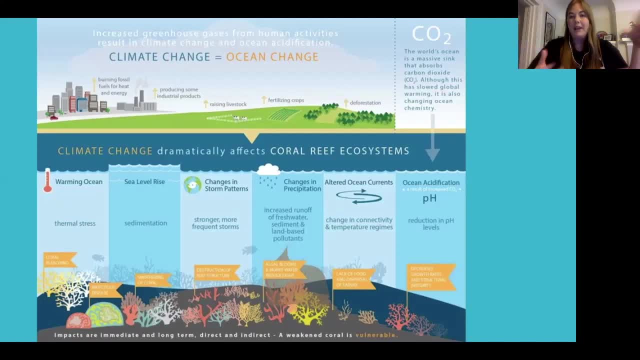 Released into the atmosphere. it is taken up by plants- Plankton, trees, corals- And so if we're cutting down trees, That means more carbon dioxide is staying in the atmosphere and going into the ocean instead of being sequestered into by trees. 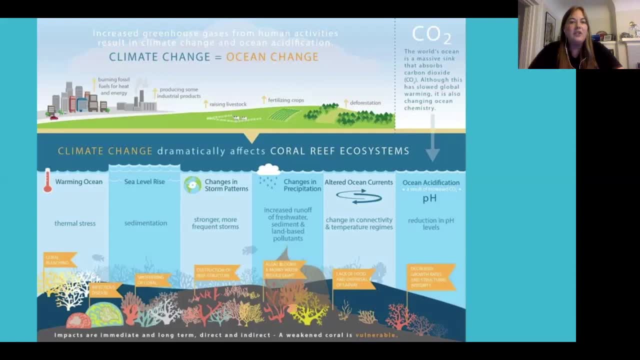 And Noah made this great graphic showing the different Variables that increase carbon dioxide in the atmosphere and then the way that affects the ocean in these different ways. So we have warming temperatures, globally Warming sea surface temperatures, which is causing thermal stress- Excuse me for corals- and then 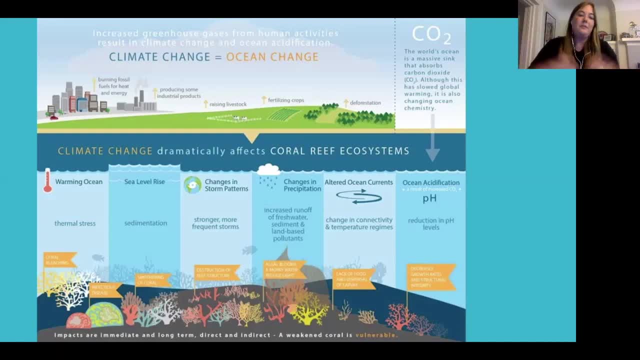 Warming also leads to melting ice caps, expansion, which leads to sea level rise And sedimentation. So as sea levels are rising, it's the water is washing up onto the land right and eroding Some of that land back into the ocean, causing sedimentation. 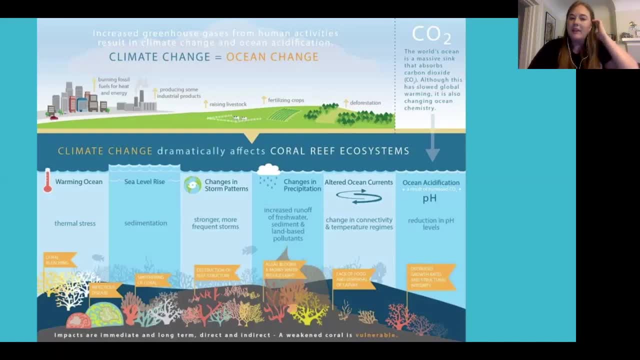 I also mentioned that we have changes in storm patterns- stronger, more frequent storms- And this also is related to changes in precipitation, So we could have an increase of runoff of freshwater, affecting the salinity of coastal habitats, Increasing sedimentation again and increasing the amount of land based pollutants that are getting into the ocean. 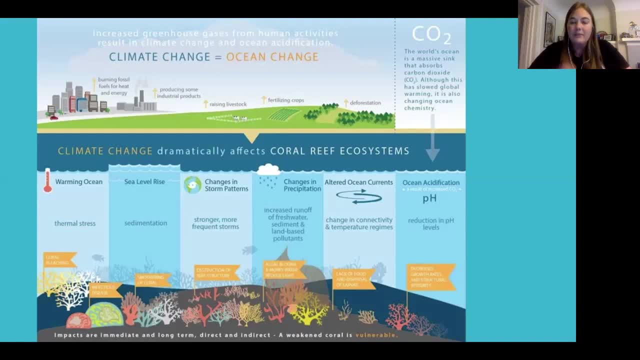 Like nutrients and other chemicals. So this leads to algal blooms And reduced light and it could, depending on what chemicals are washing into the water, it could lead directly to coral death. And climate change is also suspected to change ocean currents, which is going to have a huge effect on temperature. have a feedback on temperature and then. And climate change is also suspected to change ocean currents, which is going to have a huge effect on temperature. have a feedback on temperature and then- And climate change is also suspected to change ocean currents, which is going to have a huge effect on temperature- have a feedback on temperature and then. Will also affect the way that reefs are connected to each other. So right now, If you're born in one reef, you know as a little larva. you may travel the currents and end up in another reef, and if the current's change, You might travel the currents and end up in the middle of the ocean and not be able to surviveSo. 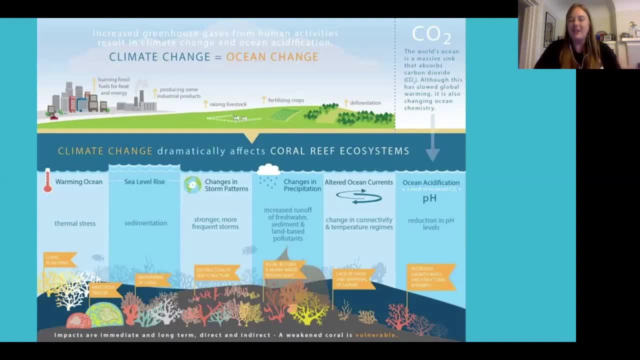 What we know now about the way that we're connected could be changing, and that changes our ability to protect reefs as well. and then, lastly, there's ocean acidification, so that carbon dioxide isn't just staying in the atmosphere, it's going into the ocean and it's 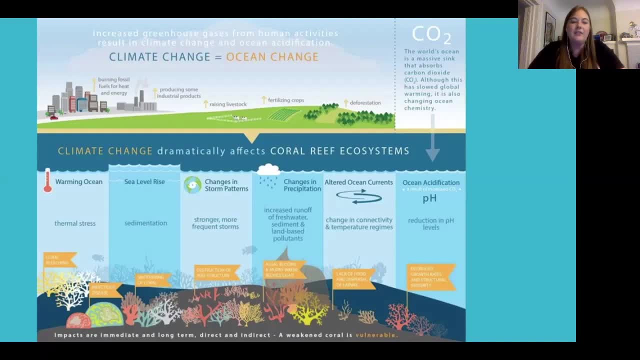 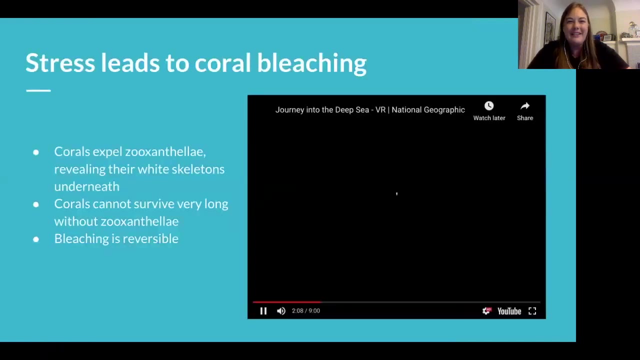 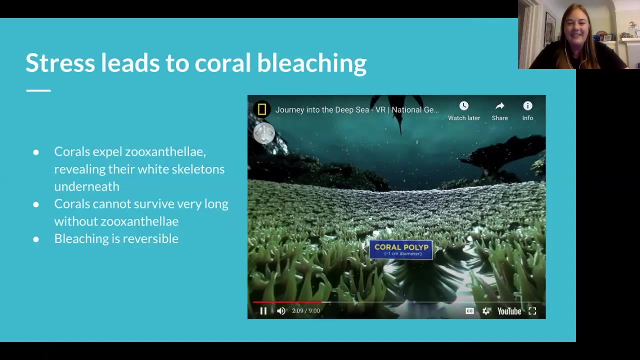 reducing the ph of the ocean, which has really harmful consequences for corals and any invertebrate. that is building a calcium carbonate skeleton, and we'll see a little bit about what else. what else um why this is so important, right? so sustained high temperatures stress out the coral animals. 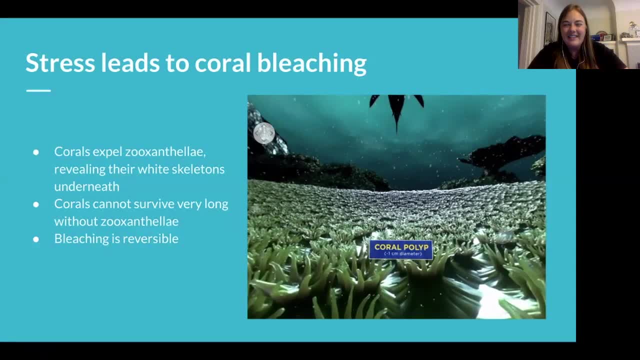 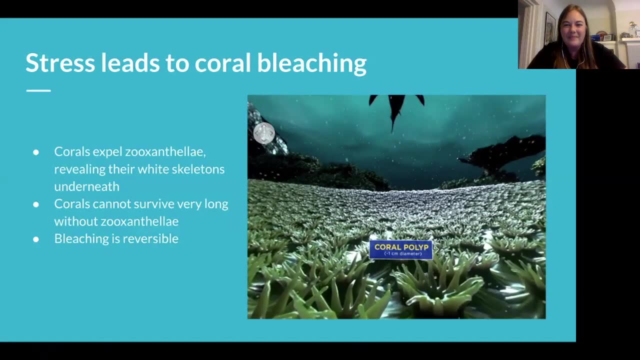 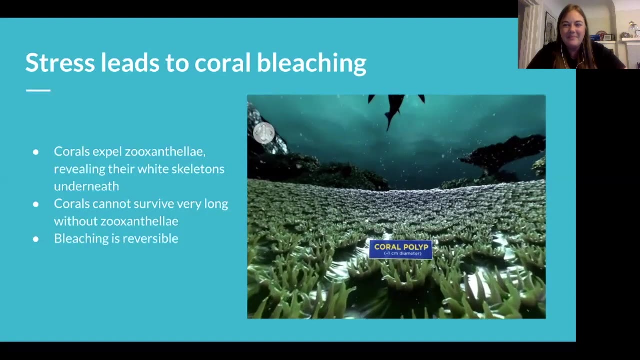 enough to expel their symbionts, which are a type of specialized algae that live in the coral tissues and provide food for their coral host. when these algae are gone, you can see through the clear coral animals to their white calcium carbonate skeleton. hence the term bleaching. 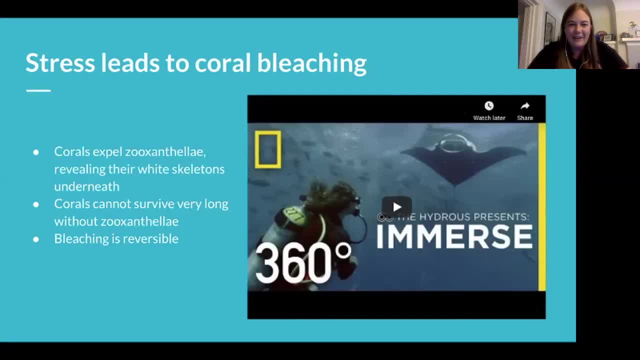 okay. so that clip from immerse was showing corals expelling their zooxanthellae, which is called coral bleaching, and this happens as a result of thermal stress but also other types of stress, and corals can't survive very long without their zooxanthellae, so this is one of the 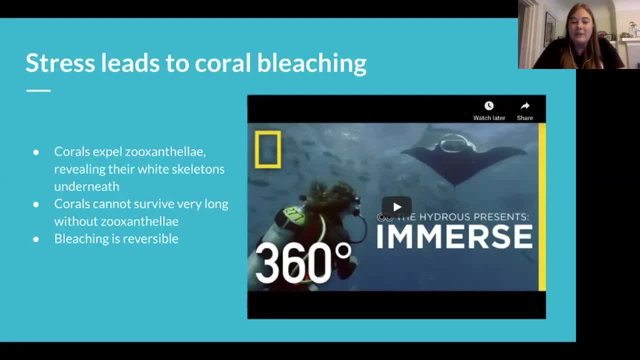 big um reasons that corals are starting to die as a result of climate change. i think i'm going to go back to that. uh, i'm sorry. i feel like i'm looking at a lot of comments in here and i am sorry. we've got a lot of time, but it's she is saying that corals can't survive. 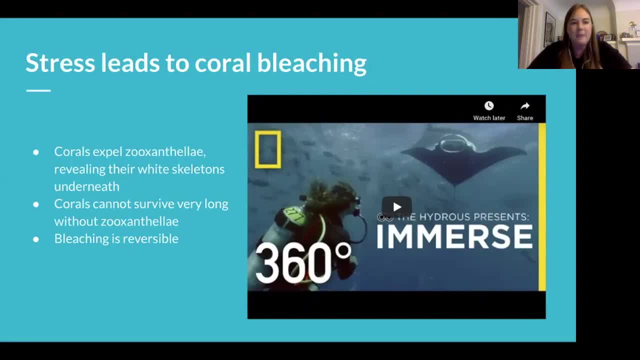 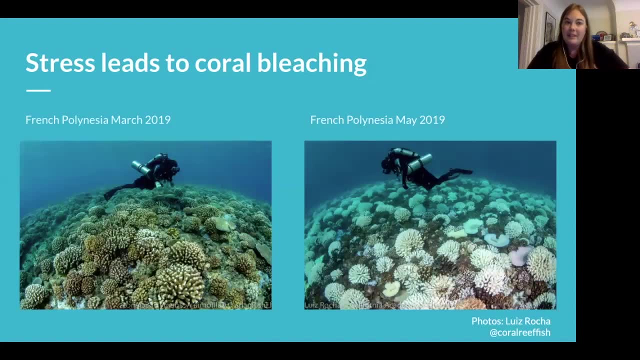 the announced that they can't survive, the things that we all think about, um. so these are the um, um perennial changes in the coral. and i did look at an actual topology study and there's a lot of information here that the corals can survive, but they can't survive the source of the stress. but it has to be, you know, the stress, whatever is causing the stress, needs to go away in order for the corals to take their zoxanthellae back in. so that's a very short time skill that that needs to happen. on um, you know, if the coral remains bleached for a few weeks or months, they are likely to die. 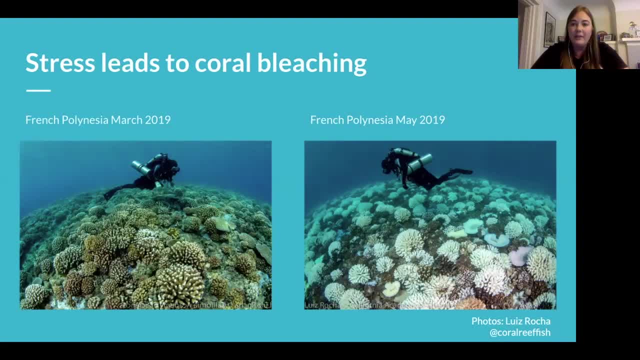 taken from by Luis Rocha with California Academy of Sciences, and so they traveled to French Polynesia in March of 2019.. Temperatures were high while they were there. They went back two months later and this is what they saw: The same reef. more than half of the corals were bleached. 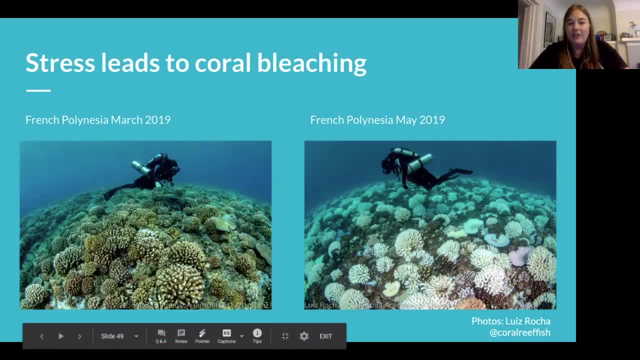 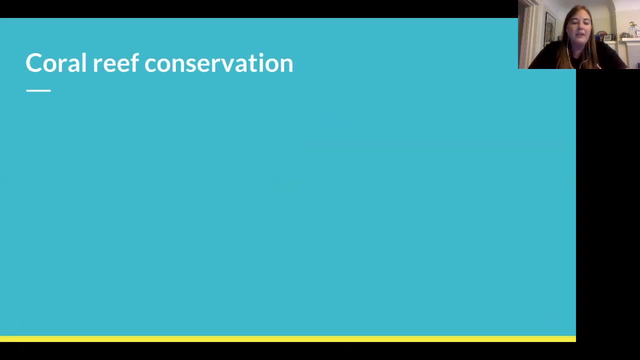 and I haven't heard yet a follow-up to see if you know if all these corals ended up dying, but there's a high chance that they did All right. so what are we going to do to protect our coral reefs? right, They're so threatened. 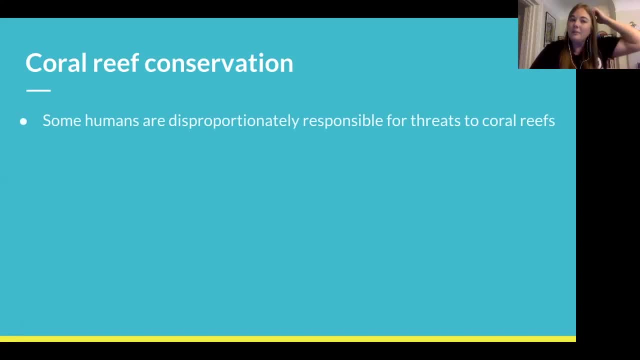 but the truth of the matter is that some humans are disproportionately responsible for these threats to coral reefs, and so they're going to do a lot of work to protect them, and so they're going to do a lot of work to protect them, and so they're going to do a lot of work to protect them. 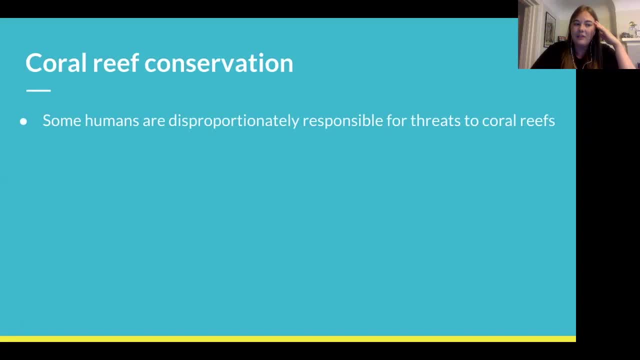 so I want you to take a minute to think like who is most responsible for the destruction of coral reefs, and just jot down what you're thinking. Pause the video so that you can take some time. All right, so some of the people that I thought about are developed, wealthy countries. 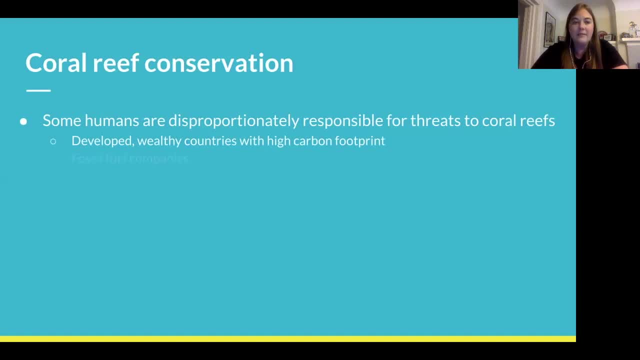 with a high carbon footprint: fossil fuel companies, large fishing companies and plastic producers and consumers. Now other humans are disproportionately impacted by threats to coral reefs. so why don't you take a minute to jot down who you think is affected most by this destruction? 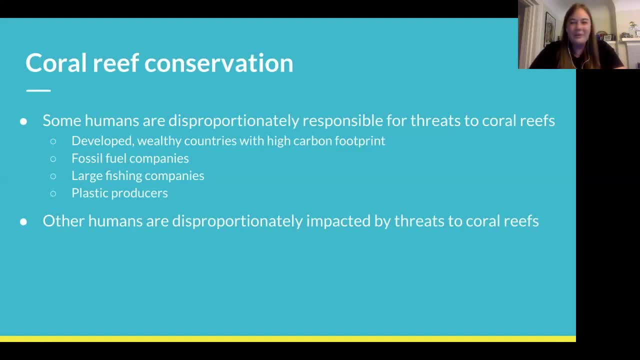 All right. so the people on my list are subsistence fishing communities, residents of the coral triangle and really any country that has a reliance on coral reefs for the economy, be it through tourism, the aquarium trade or fishing. there's a lot of people that are really reliant on coral reefs. So I want you to hear just a little bit of what's going on in the world right now. So I want you to hear just a little bit of what's going on in the world right now. So I want you to hear just a little bit of what's going on in the world right now. 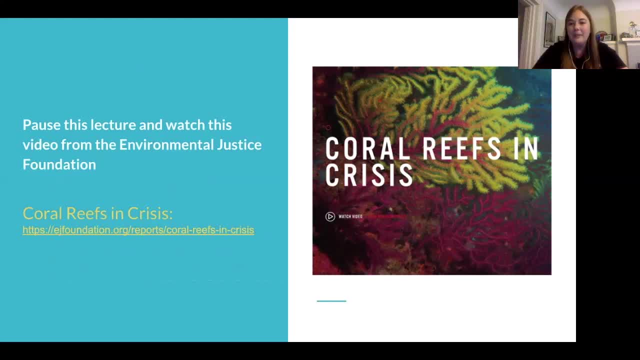 But I want you to hear directly from these people because you know I'm I'm safely, you know I'm not protected from climate change, but I'm, but I have. I'm coming from a privileged position, right like I love coral reefs, but I I'm not as directly connected to them as a lot of people are in the world. 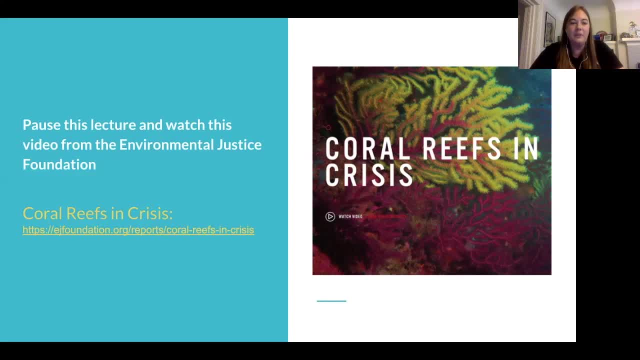 And so I want you to hear from from someone who lives in the area, in the area that really, really relies on coral reefs, and so I'd like you to pause this video and go to the Environmental Justice Foundation's website and watch their video on coral reefs in crisis. 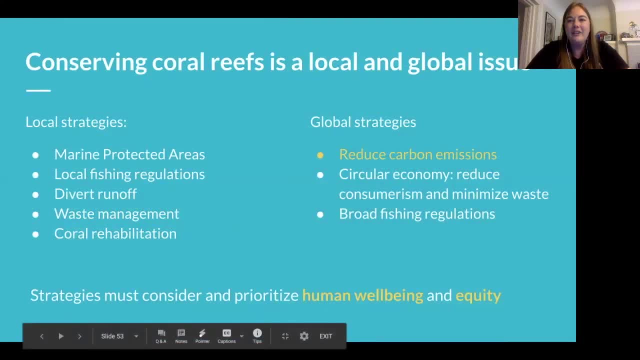 Okay, so coral reef conservation is something that can be tackled locally and globally, and so I'm not going to go into all the different strategies, but I did want to highlight the fact that the main threat that we have right now is climate change, right? so the thing that I think that I'm prioritizing, focusing on 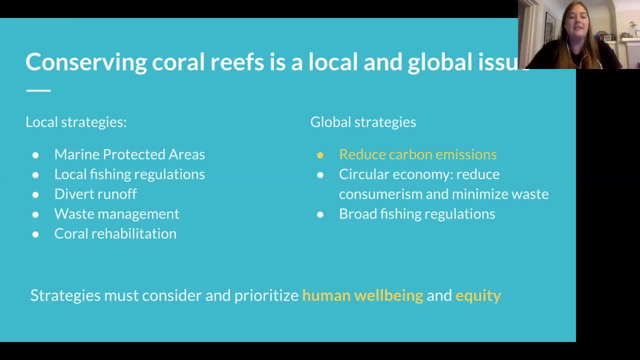 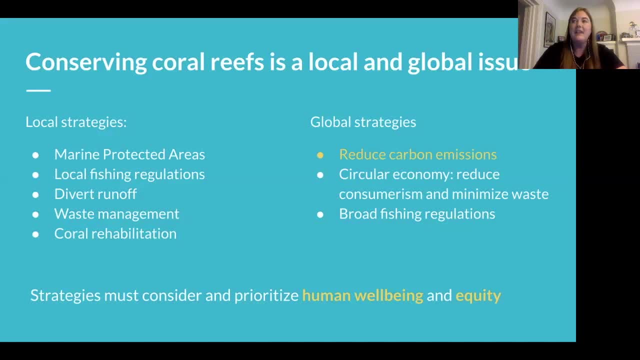 involved. I just wanted to point out that it's really important that these strategies consider human well-being and equity in design of whatever conservation intervention you're planning to do, and so I really liked how, in the marine marine conservation lecture, Dr Chelsea Crandall said this. 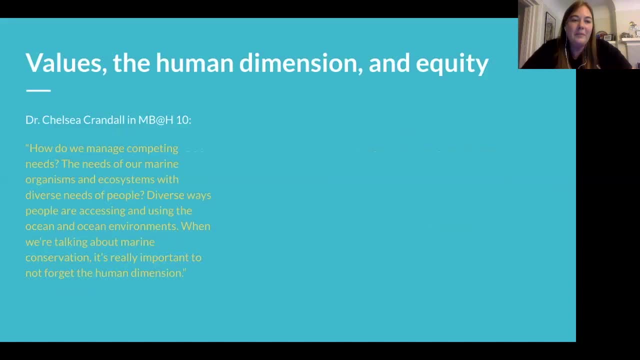 how do we manage competing needs, the needs of our marine organisms and ecosystems, with diverse needs of people, diverse ways people are accessing and using the ocean and ocean environments. when we're talking about marine conservation, it's really important to not forget the human dimension and one of the examples that 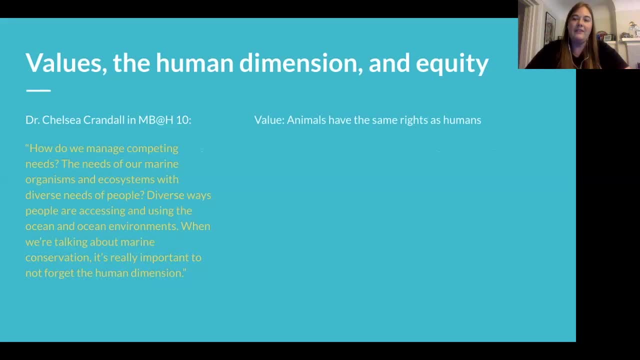 Dr Crandall gave, was this sort of value and attitude relationship between the two Add damaging to your fishing environment. does a part of however we worry that is so just to rephrase these his comments are. So the example she gave was the value that animals have the same rights as humans. 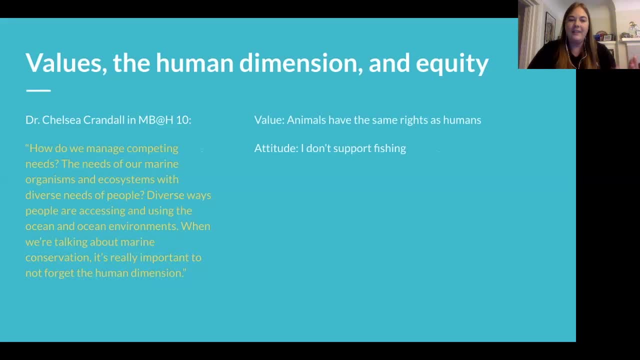 And then the attitude that could result from that would be that I don't support fishing. but Dr Crandall was pointing out that we need to think about the complexitiesでは荻人 savoir Doctor Crandalloléote oqëjções Re答? term Xiao animales úr. human dimensions. So here we have to remember the here we have to remember that there are people whose survival is directly dependent on fishing. Okay, So in those cases it's really hard to say, and normally I take in-planting when an animal does not eat, so that you're only roaming in the ocean. 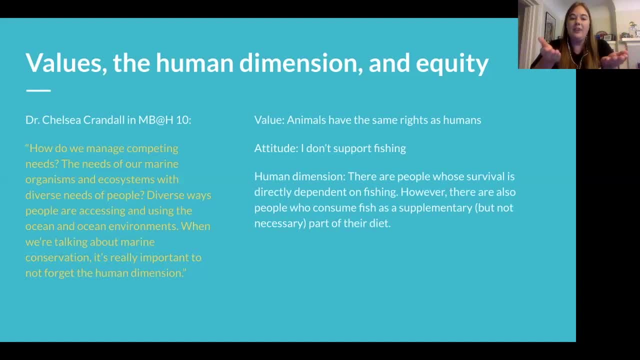 Okay cases, it's really hard to say, well, just don't fish, because then you're actually valuing fish over humans instead of having equality right now. on the other hand, there's people who consume fish as supplementary to their diet, so they're not relying on fish, they're just choosing to eat fish because they like. 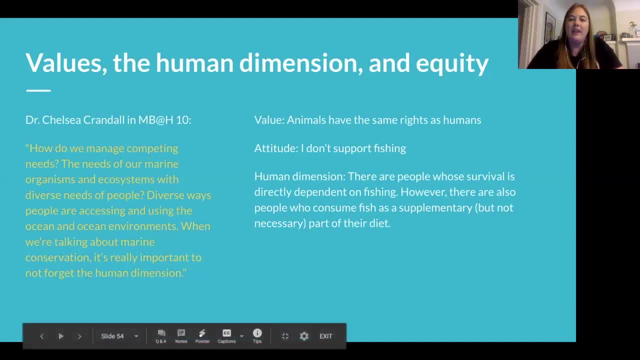 it, and so an equality lens might say: well, we need to. we should treat all people the same and have the same policy around the world. but that can lead to inequity, because fishing restrictions will have a disproportionately negative effect on the people who rely more on fishing right, so you can't have the same. 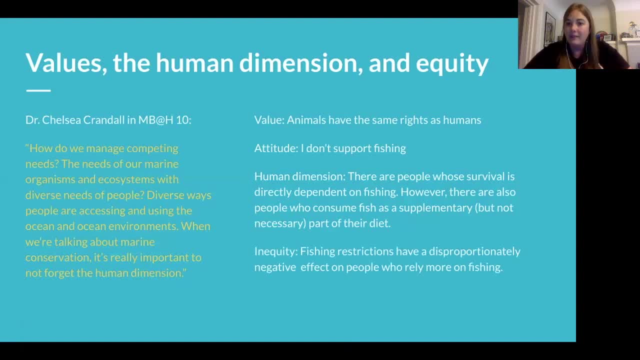 rules apply to everyone, because certain people are going to be hurt by those rules more than others, and so a more equitable conservation intervention would be to restrict fishing for some, but retain the fishing rights for those who need it most, and so this is just one example. I'm not an expert on marine conservation. 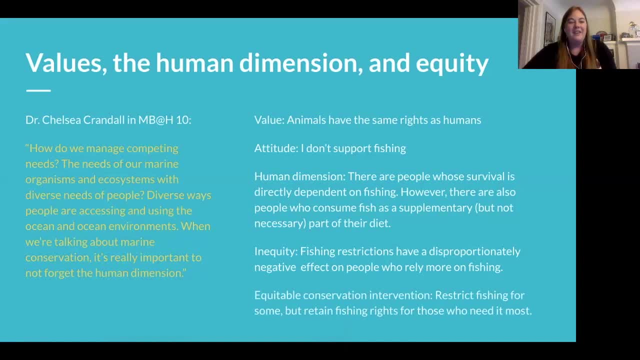 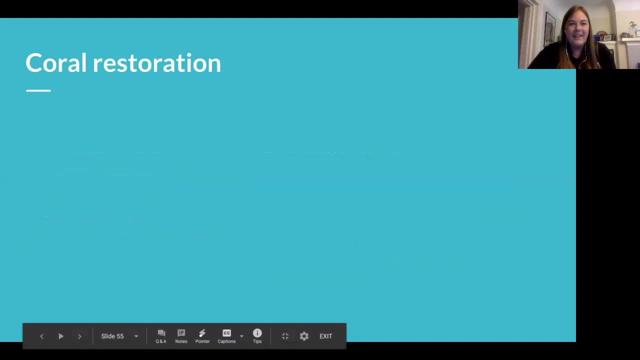 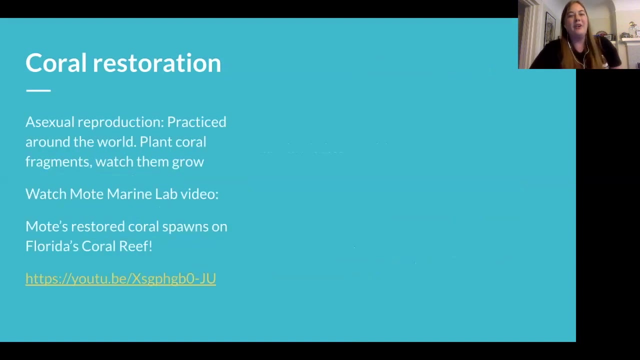 and equity, but I just wanted to make sure everyone is always keeping that in mind right now. some of my favorite conservation stories right now are about coral restoration. so I encourage you to look at this story about asexual reproduction, where people who have basically planted fragments of corals that are now growing and thriving and spawning. so there's 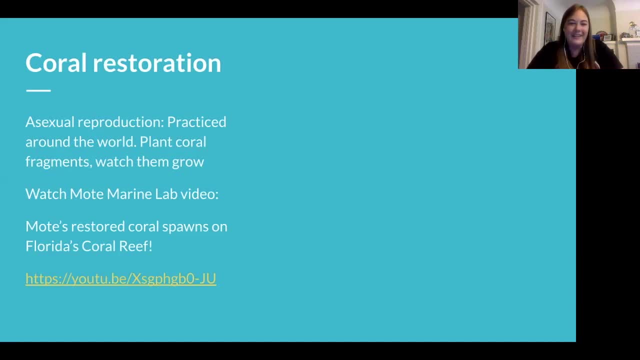 a little video about the Mote Marine Lab in Florida and how their corals are doing, and then another great one is a story of helping corals with sexual reproduction. so Seacore International facilitates sexual reproduction by collecting gametes and fertilizing them in the lab and growing the larvae, and then, once they're, you know, like thriving little corals. 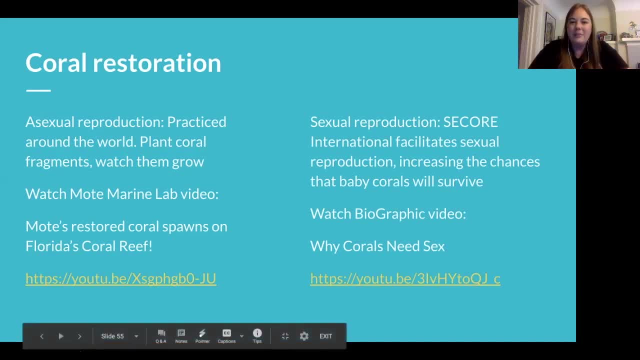 they'll put them out into the water, and there's a great video about this made by Biographic, featuring Dr Raphael Ritson-Williams, who is one of your other lecturers for this course, and yeah, it's called why corals need sex, so highly recommend that you watch these two videos for a 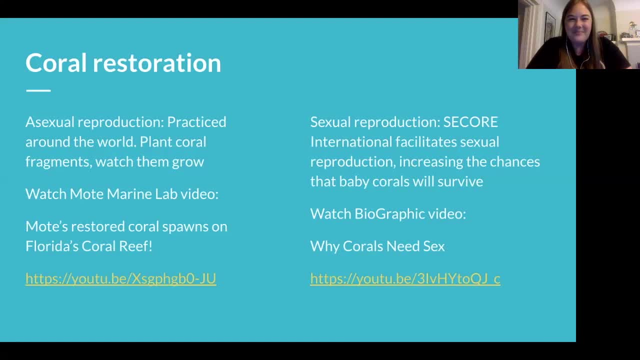 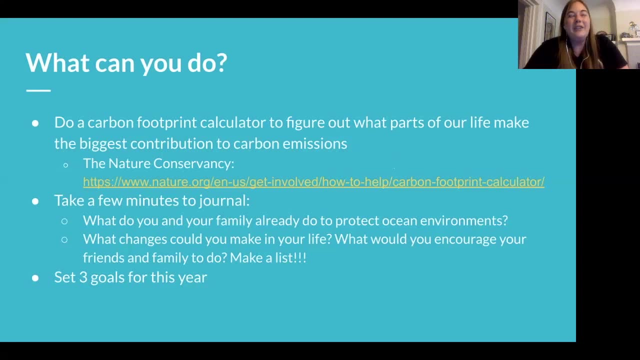 little inspiration about coral restoration and if you're feeling you know you like you want a little bit more hope and you want to know what else you can do to help corals, I definitely recommend that you do a carbon footprint calculator. figure out what parts of your life are making the biggest. 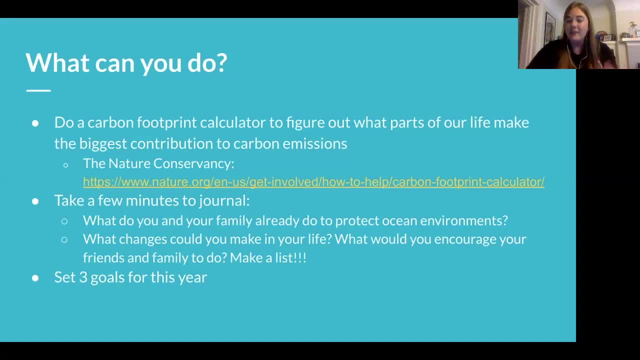 carbon emission impact. so for me it's travel, especially as a marine biologist. I've done a lot of traveling in my life and you know flying driving are huge carbon emitters, but for you it might be something different. so I like this one from the Nature Conservancy. it's really detailed. 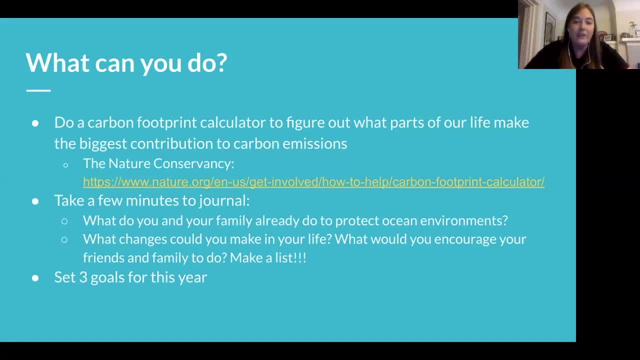 you fill out like every detail of your life and it tells you how you're doing with your carbon emissions and then you know. once you've done that, I'd say you know, to take some time just right out and see if there's anything that you would like to know about the corals and the life of the corals and the life of the corals. 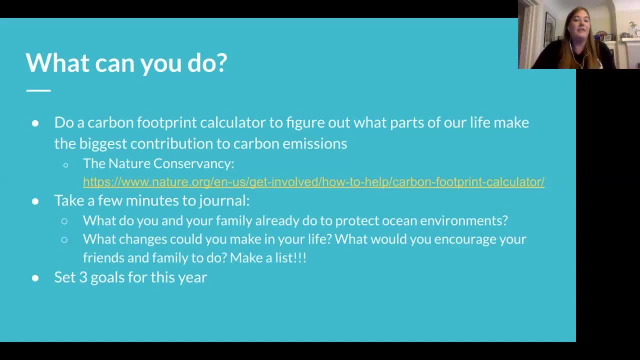 what you're thinking like, what are you already doing to help ocean environments? um what? what changes could you make or what changes could you encourage other people to make? right and make a list of all the different options and then choose three, three goals that are um attainable. 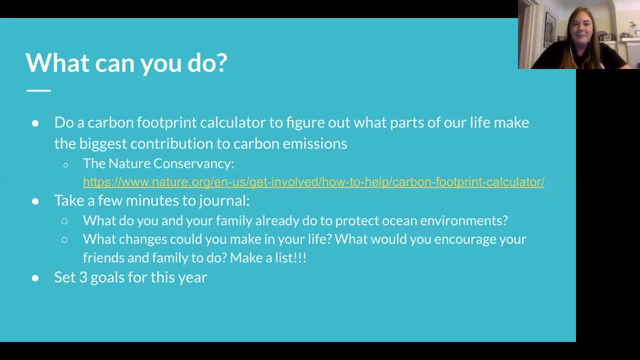 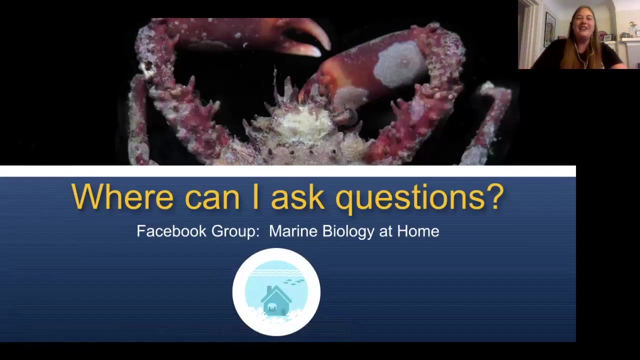 and measurable, and you know, write them down, commit to them, tell other people that you're doing it and maybe all together, we can save corals. right, that's, that's the goal, that's the dream. so thank you for- uh, you know- taking part in this class and and following me along on this journey. 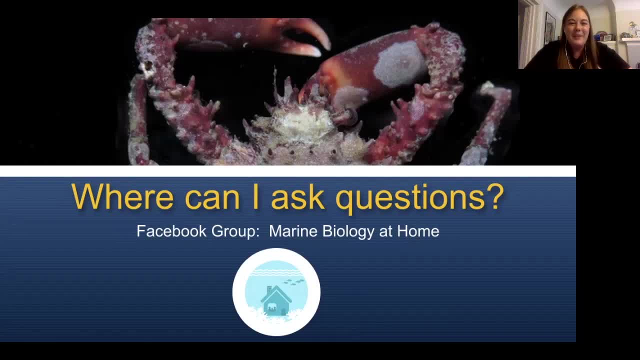 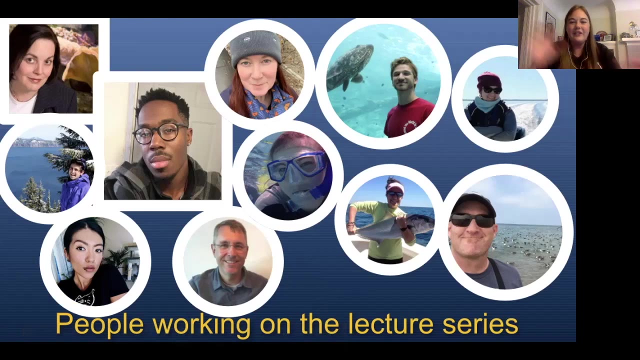 through coral biology and ecology. um, if you have any questions, please visit the facebook group marine biology at home. i'm there, um, you can tag me if you want to answer questions. um, i also want to just acknowledge everyone else who is contributing to the lecture series. it's 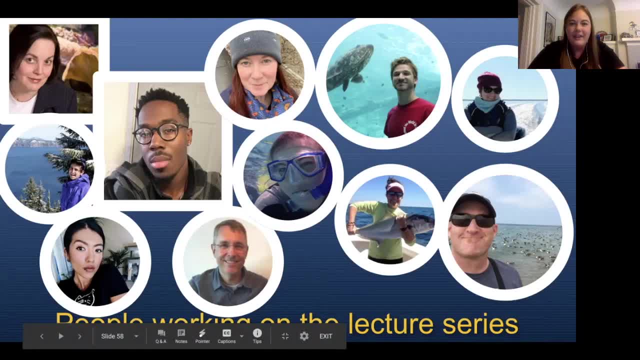